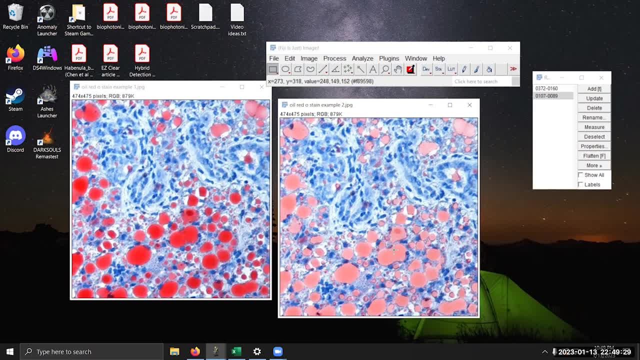 this could lead to substantial problems in interpreting those numeric results. Let me show you what happens and how we interpret it. In particular, I want to showcase multiple approaches that people can try and give my critiques about how they do or do not work for this color. 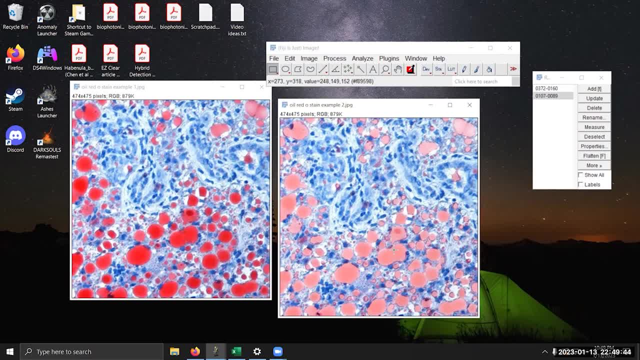 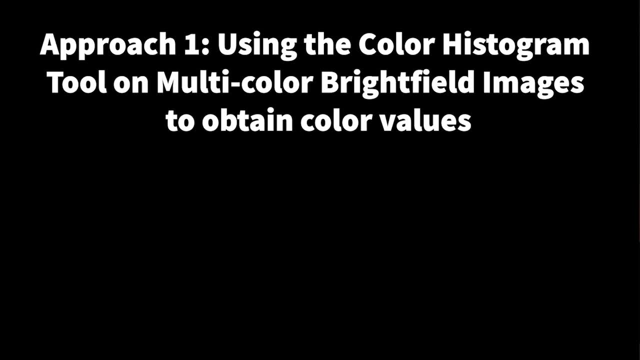 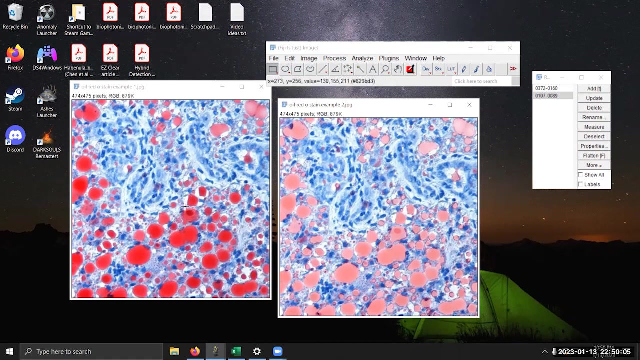 comparison goal you may have. First we'll start out with what I'm calling approach one, Approach one, Using the color histogram tool on multicolor bright field images to obtain color values. Verdict Works, but not ideal. So in our normal stain window, select an area of interest. I chose one red blob. I had already. 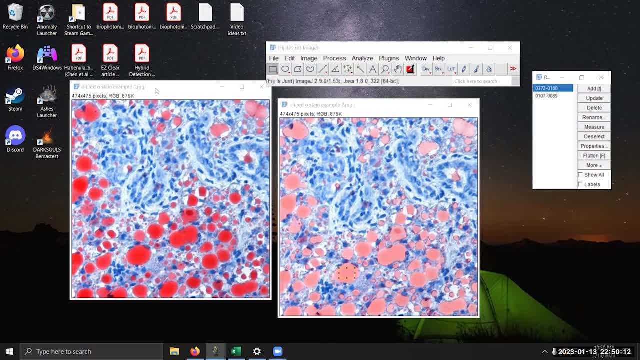 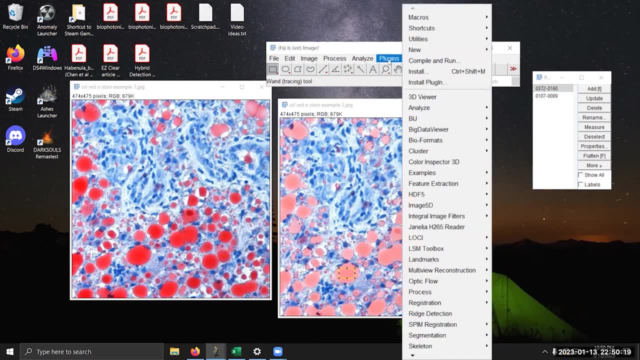 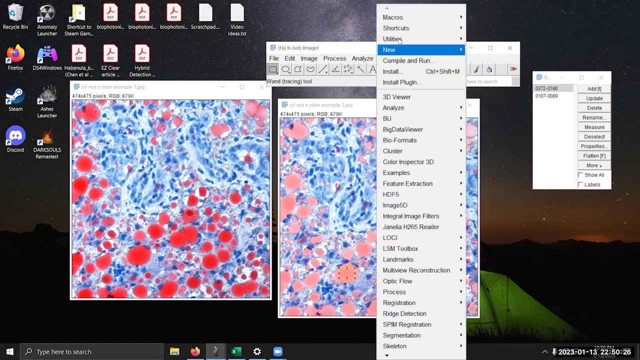 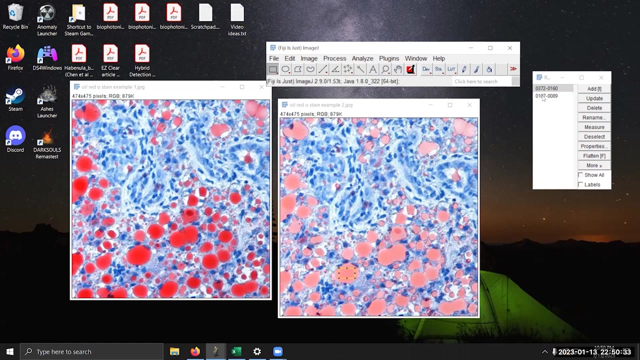 added this selection to the ROI manager. Now to get the ROI manager, I believe you can go to plugins, tools, or it is under one of the tool menus in here. You'll have to hunt around for it. I've already added this to the ROI manager so that when I click on the window and then I click. 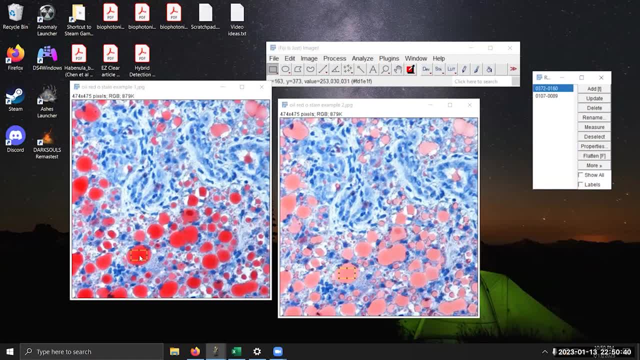 on this specific selection. it pops the box right into this red blob down here. We see that it did also the same thing for the exact same location in the other image of the faded stain. So I did this thing through the ROI manager to make the selection boxes the same size, same location, to. 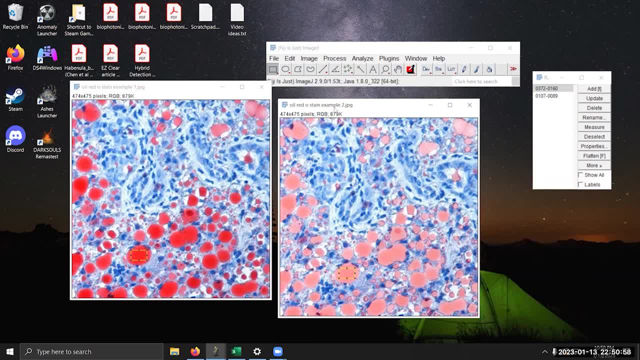 keep things as consistent as possible for the purposes of this video, to show you how we can compare the numbers. However, for your applications, you don't necessarily have to do this. The box sizes don't necessarily have to even be equal between two different images you're comparing. 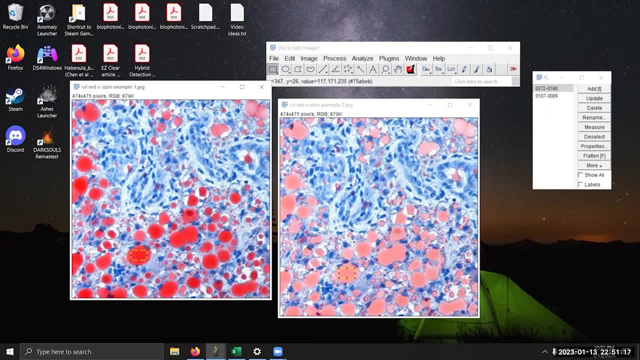 So we'll start off with the normal stain, Select the normal stain image- while being careful not to click on anything within the image that might alter the selection box that you've drawn- and go to analyze color histogram. So this pops up a few results here. 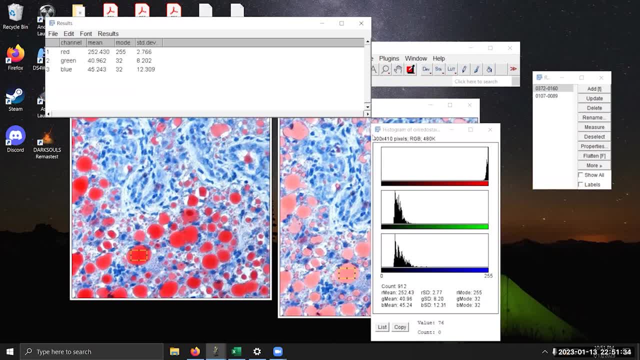 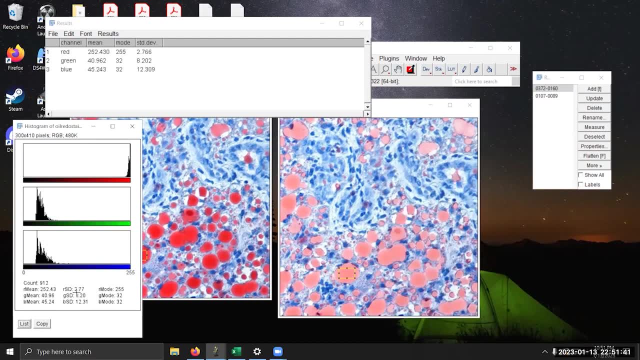 You can copy things as results box into an Excel spreadsheet And we also are given the actual histogram data. that gives us also the same numbers at the bottom here. After you've copied down the data from the results window, you can then click on the other stain that you want to analyze this. 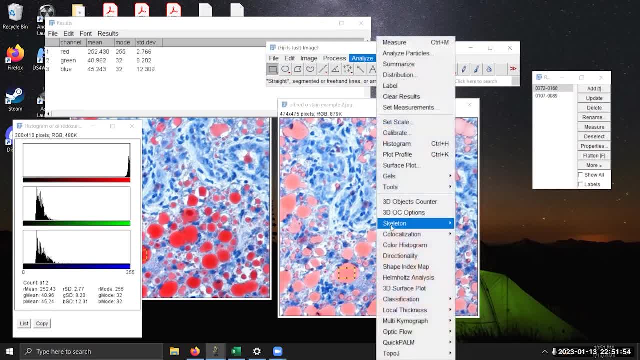 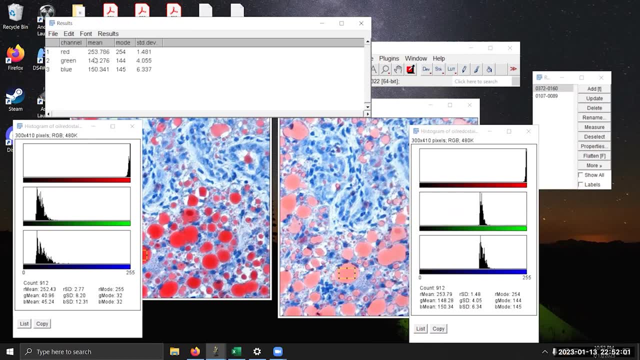 faded stain in this case- and do the same thing, analyze color histogram. You'll notice that it refreshes the values here in the results window. It overwrites them. So you can see that the results. So it's good to copy them down before doing the color histogram function again. 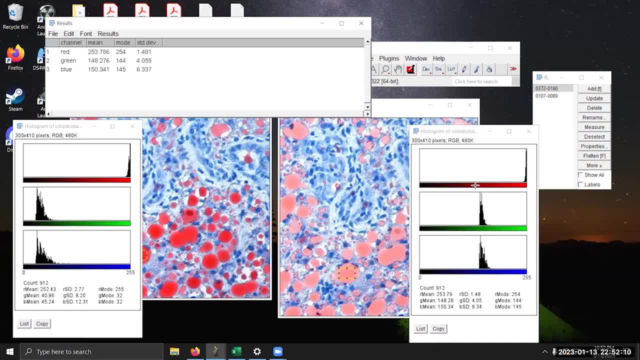 Looking at the histogram windows, we see that there is some variety of the colors they sample, And we could figure this out by the color curves. Basically, it's not one steep spike, but instead actual curves of colors. Now, looking at these results, you might be tempted to just compare the R mean for the red mean value- 252, versus the R mean of the other one, 253.. 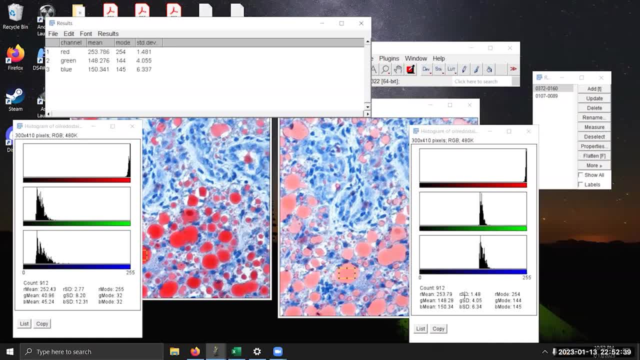 However, this is going to be a wildly inaccurate comparison based on how much the other two colors, green and blue, contribute to the actual coloration of the multicolor image. So this might seem odd. Why is it that the blue and green values are so different? 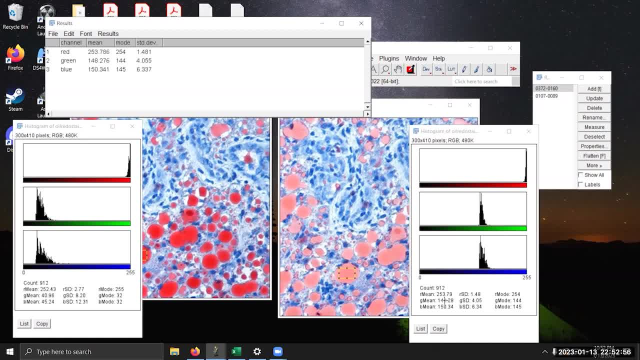 Why is it that the blue and green values are higher than zero for these selections? since I only selected things within the red blob, I didn't pick up blue or green. In other words, why isn't red the only notable or major color that has a value here? 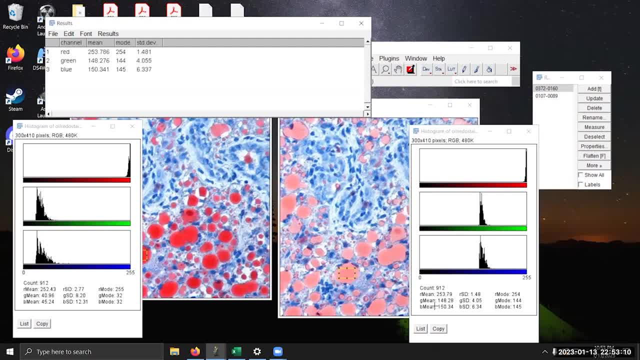 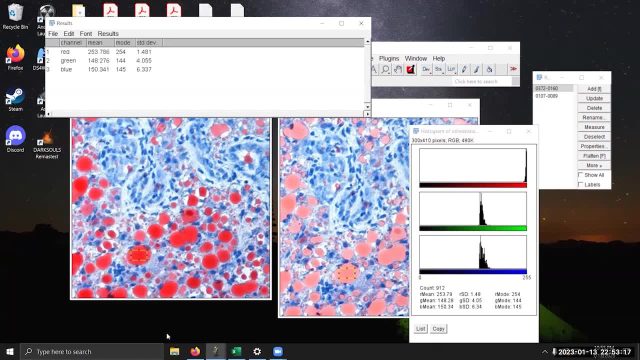 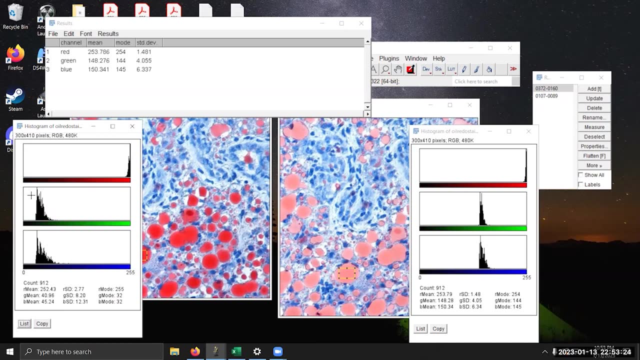 How are these values for blue and green so much higher than zero? Well, to figure this out, let's look at what the color ranges are for each color. Looking at the color histogram boxes specifically, Oops, You'll notice that The color histograms, they start at zero and all of them are black for each of these colors. 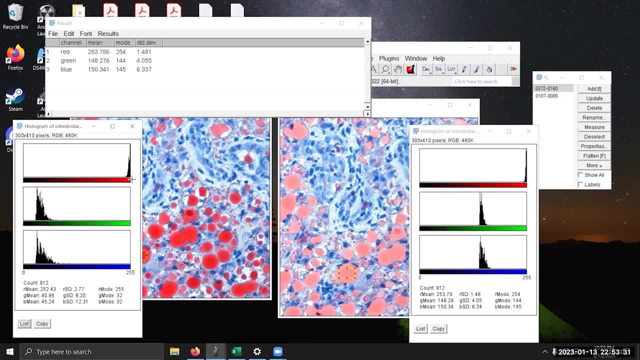 When they go to 255, they are their true or pure color And the issue is that when we add all three of these colors together, when they're at their maximum, in other words, 255 is the purest red, 255 here is the purest green, 255 is the purest blue. 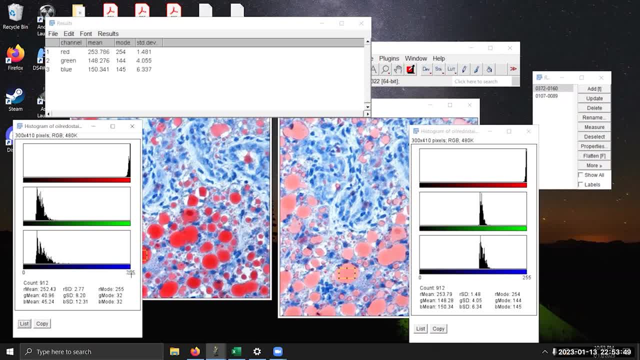 When all those are added together they create white. So in order to get white or any sort of intermediate Colors, there has to be a combining or an addition of these colors in these different channels. So we see these massive shifts. then, when we look at the comparisons within the selection box and the normal stain image, we actually see numbers of for green, of 40 and 45 for blue. 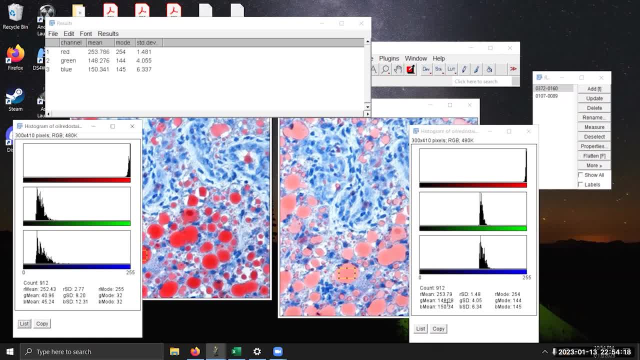 And then we compare those for the faded stain and we see 148 for a green and 150 for blue. So the numbers for blue and green are much higher. In other words, we're looking at the same thing. In other words, they add with the red to bring it closer to white. 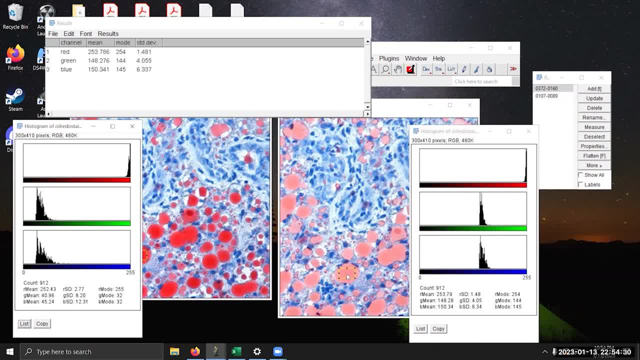 That's why the stain looks faded, because it's actually closer to the background color, to white, and less red. as a result, When the numbers for blue and green are lower, then the red sort of shines through. It's not mixed with these other colors that bring it closer to white. 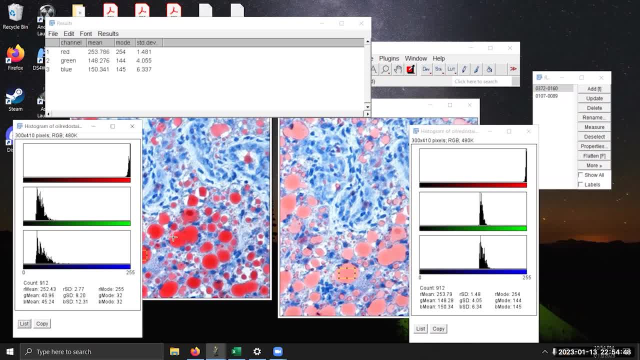 So that explains why on the left-hand image it's more predominantly red and that the green and blue have much less of a factor in that. So we cannot just compare the red values, as it substantially overlooks how much green and blue are involved with how the color histogram analyzes staining intensity. 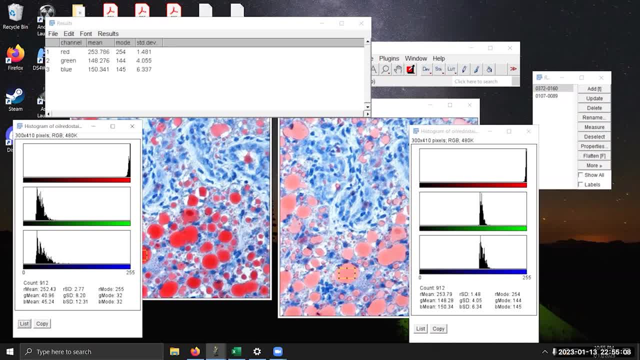 One approach could be that you check how much your color of interest changes. In that case, the color of interest is red and it changes minimally. Then you can compare the mean values for blue and green respectively, So in other words comparing 40 versus 148 and 45.. 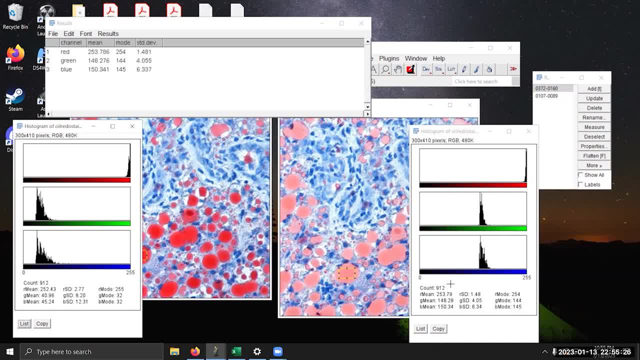 Now, although this approach can work, it certainly makes the analysis non-intuitive. Also, this approach for just using the color histogram function on a multicolor image does not account for cases in which your stain may change color. For instance, a bad stain may not be faded like the red one shown here, but it actually may be a different color entirely, like, let's say, purple. 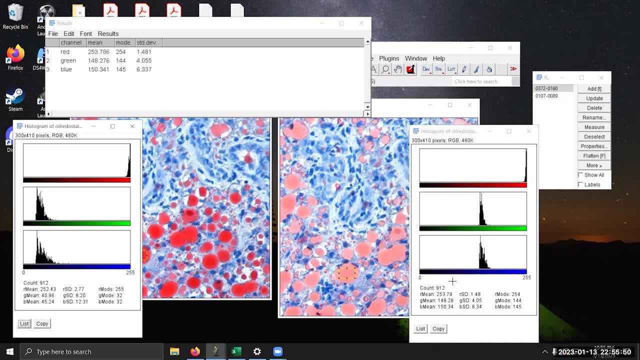 In that case it may be in your interest to compare all three values, with the knowledge that they all combine into white when they're left-handed. So you can see that the color levels are high enough collectively. All right, so that's approach one. 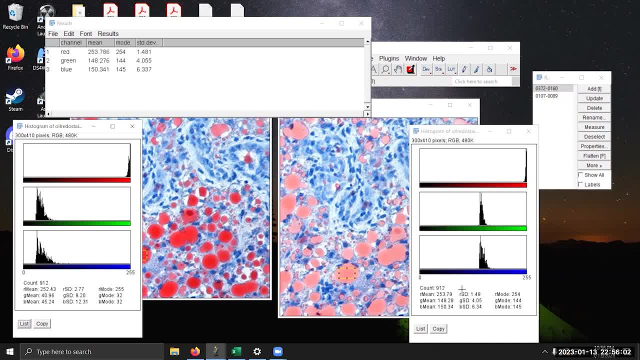 Since this first approach might not work so well due to its complexity and complication, the next option we should consider is how we can measure isolated channels of the image. We can actually split the colors up and just try to use the same color histogram tool on the isolated color channels. 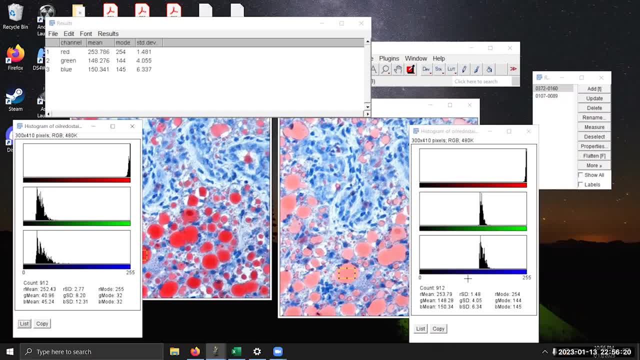 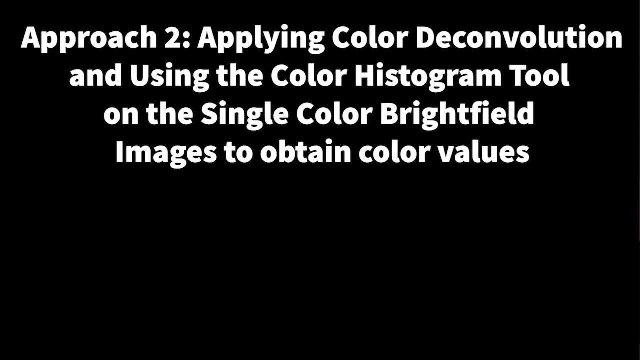 In this case, you'll see why that might not work so well. still, Approach two: Applying color deconvolution and using the color histogram tool on the single color brightfield images to obtain the color values. My verdict Not recommended. So how to do this? 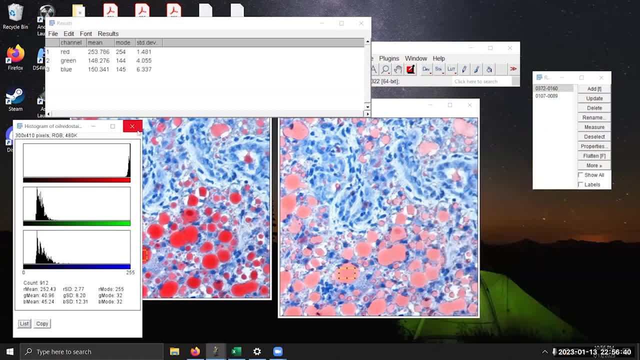 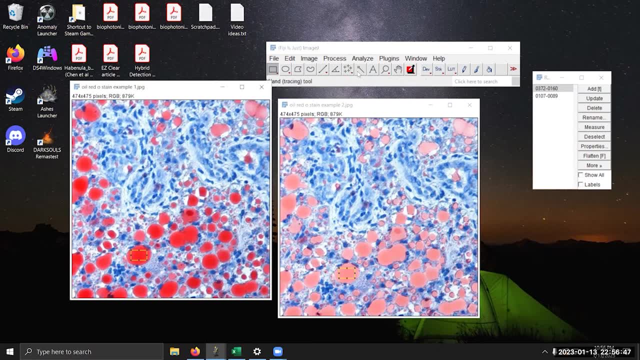 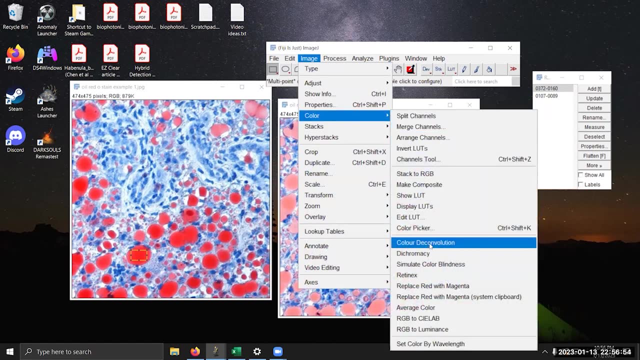 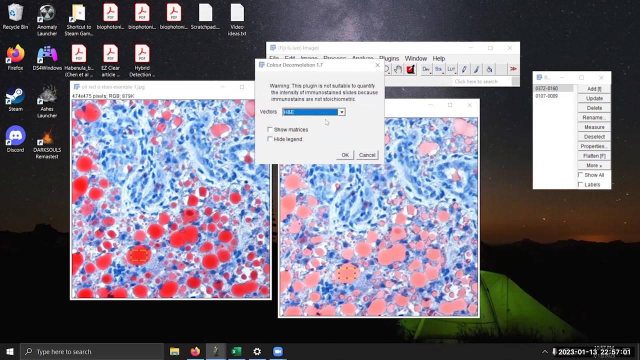 Well, we can clear out the original color histogram windows. Minimize this for the moment And we'll click on the first image. Go to image. Color Color deconvolution, Since there is not a Oh quick aside here. 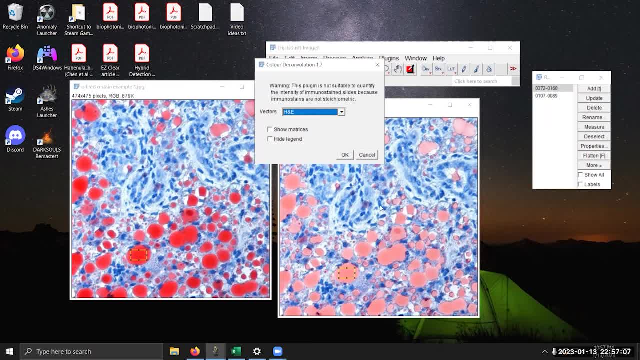 Please note that if you don't have the color deconvolution as an option, you may need to find and install the most up-to-date version of Fiji, That is F-I-J-I, Because that's the one. that is the version of ImageJ that has a lot of the plugins, such as color deconvolution and a bunch of other things. 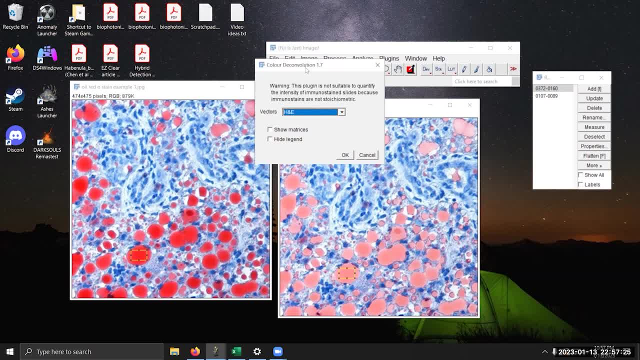 You'll notice in the color deconvolution dialogue that there isn't a specific setting for oil, red O stain Or for whatever the counter stain here is, So I'm deciding to divide it into red, green and blue. 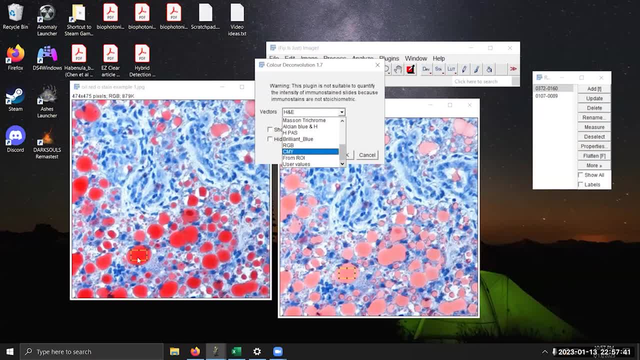 We can kind of look at the stain and see that, oh well, sure, the red and the blue separate, And if they were green it would probably stand out relatively well too. So I'm going to check the RGB setting. 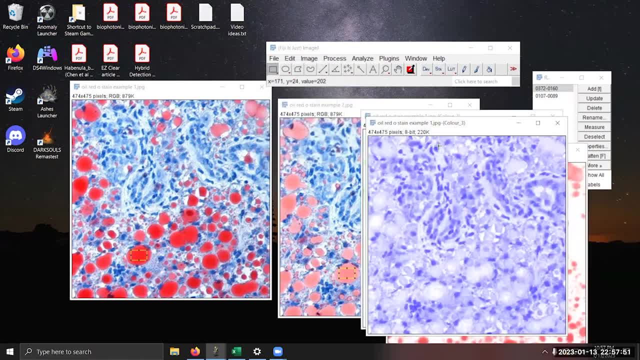 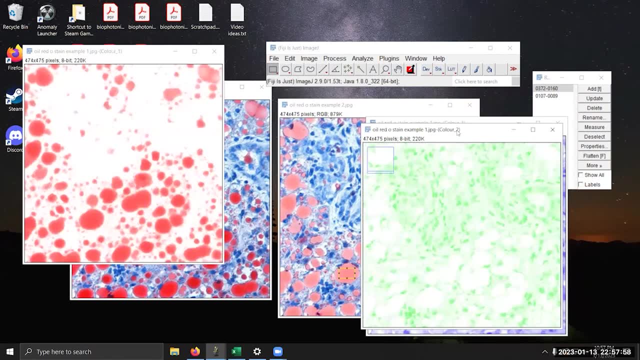 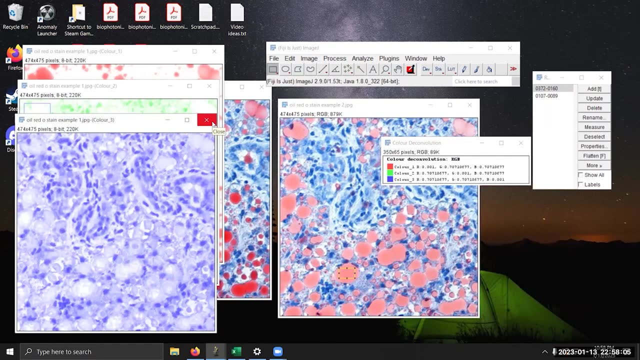 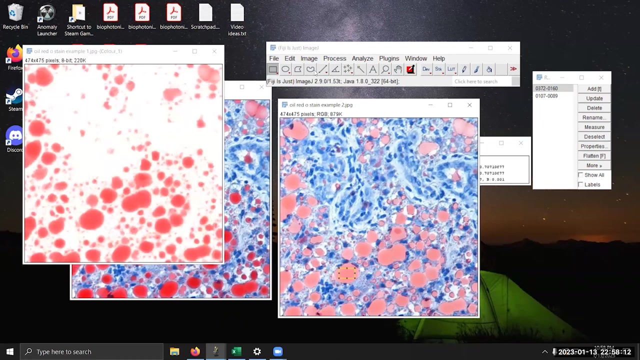 And then I will hit OK. It creates these three images here. that are the separated colors. We can see red, green and blue. For now and for simplicity's sake, I'm going to close these other image panels. We can also deconvolute the other image, the faded stain. 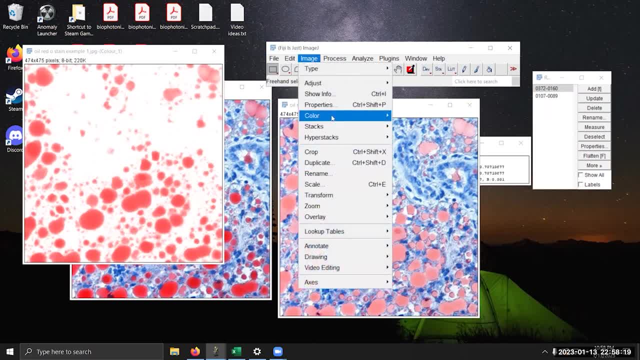 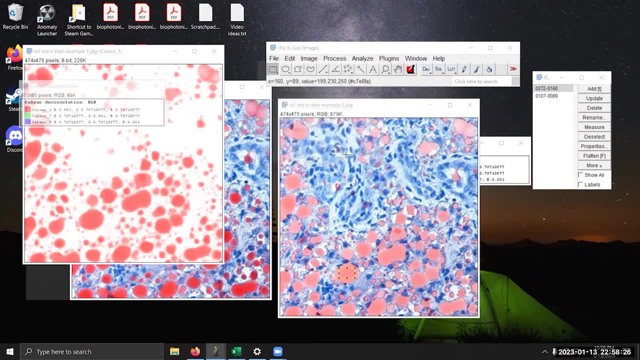 So same thing. We go to image color deconvolution, Select RGB from the dropdown menu, Hit OK And again we get a whole collection of images Going to cut out blue, going to cut out green and keep the red. 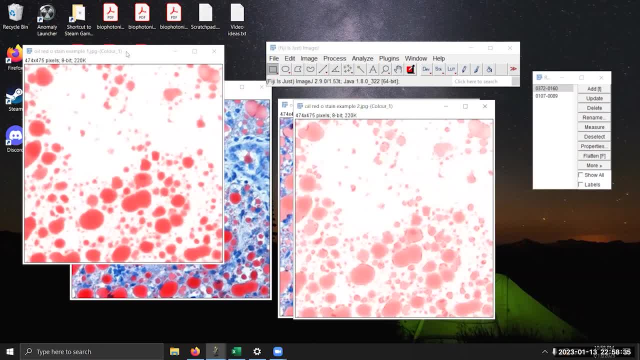 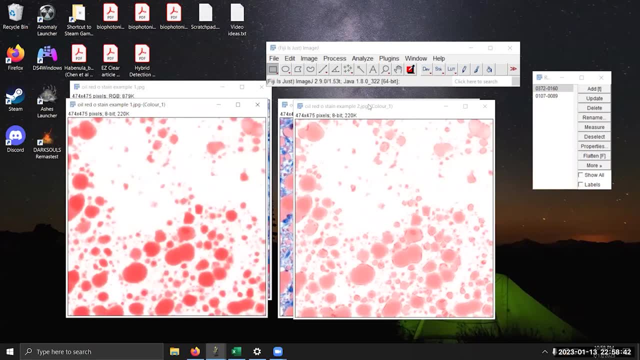 When we look at the reds side by side we can see the fading effect. So we know that we've isolated the red here. Let's say I try to do the color histogram again First. before I do this, I need to redraw the selection. 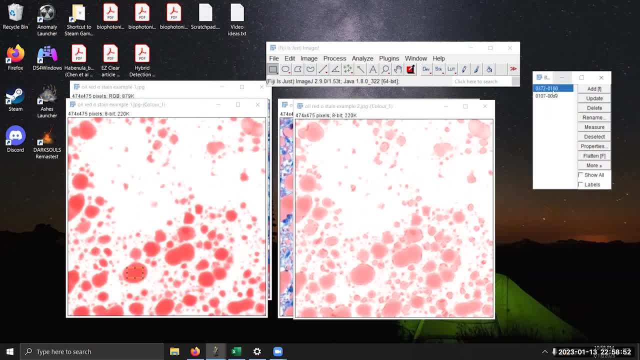 So I'll just go back to the ROI manager. Click on the window. Click here: Redraws the box there. Click on this window. Click here Redraws the box there. Now, if I try to do the color histogram analysis on it, it'll give me this error message. 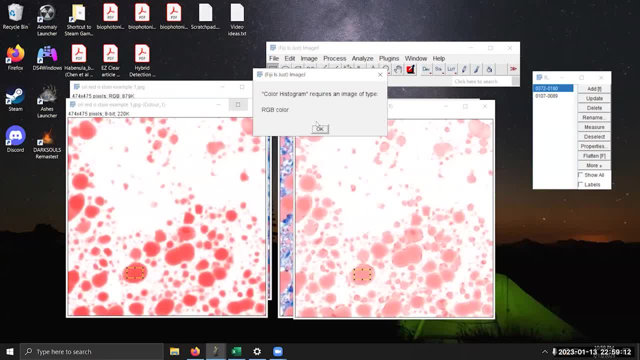 And you'll notice that it'll say that we can't do this on this image. We need an RGB color type image So we can convert these images into RGB color To make this approach work, This approach number two. So let's go ahead and do that. 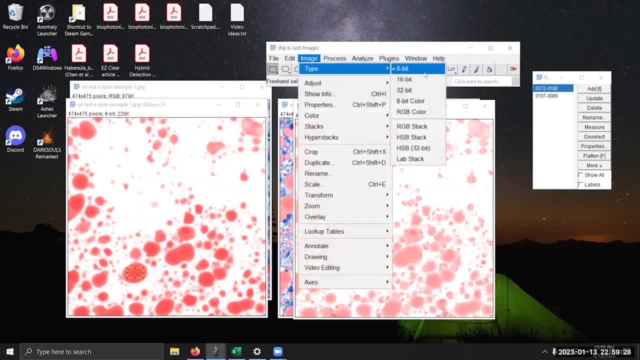 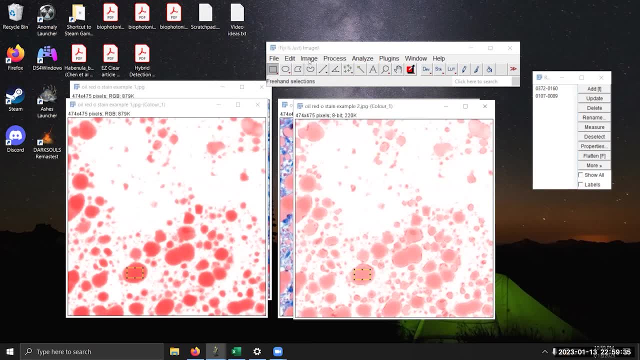 We can go to image type and change it from 8-bit to RGB color. So that has converted the image type. We do the same thing for the other red, isolated channel Image type: RGB color. Now we can click on these and again populate the color histogram. 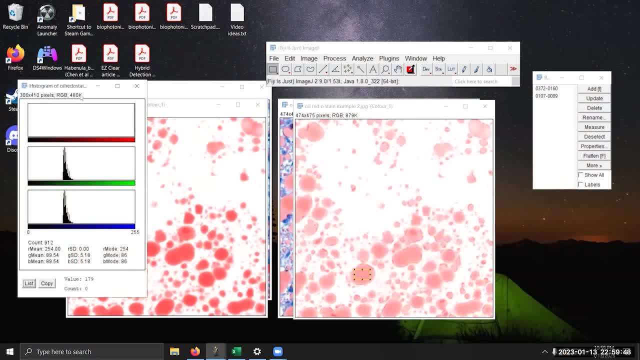 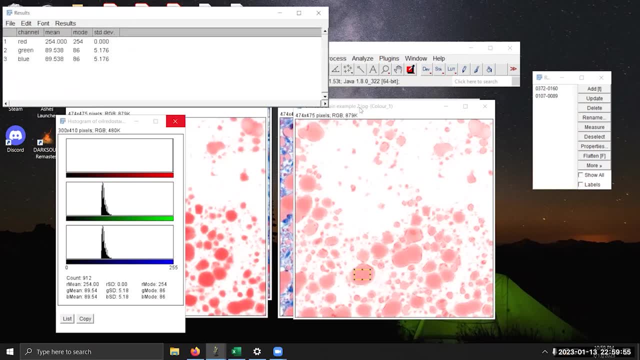 So let's go ahead and do that. So we have this here again In the results window. you can copy over the data into an Excel spreadsheet And then we do the same thing over here: Analyze color histogram for the faded stain. 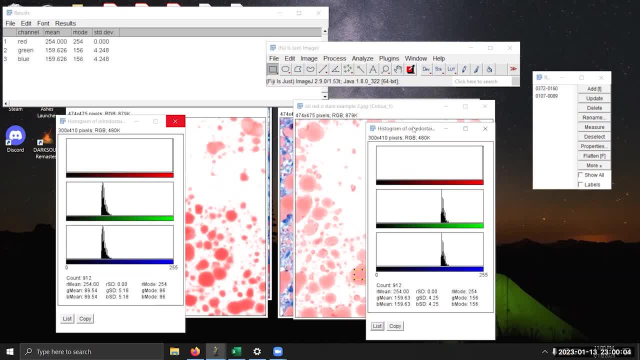 Looking at the red mean, we see that in both cases it's effectively at maximum. It says 254 here, 254 on the other one. That again seems not so intuitive, Because the red looks like it's changing, because it's faded. 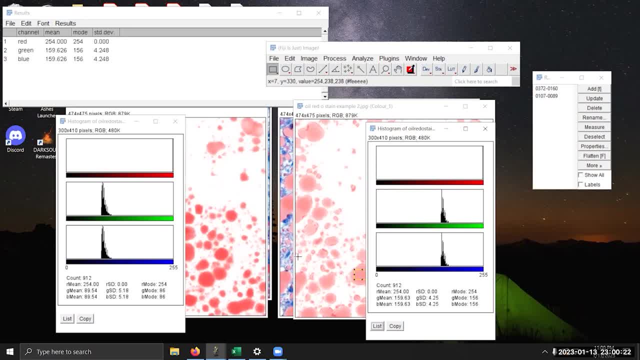 But we have to remember it isn't the red value that's changing, But the other values that contribute, bringing it to closer of a white color. So then, how do we measure it? Well, we have the same problem that we did before. 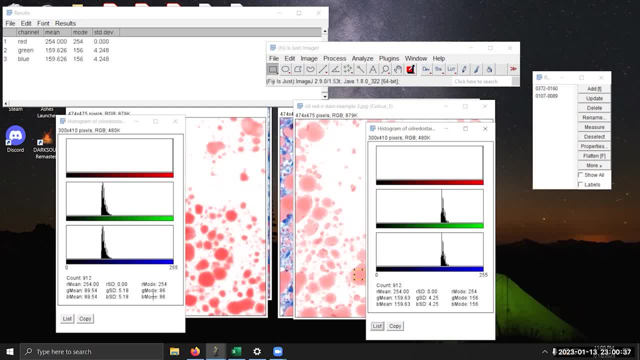 We have to look at the green and the blue values and measure the difference therein, So green versus green, blue versus blue, 89 versus 159 in these cases. All that said and done, These previous approaches may give the impression that the color histogram tool somehow overcomplicates your analysis. 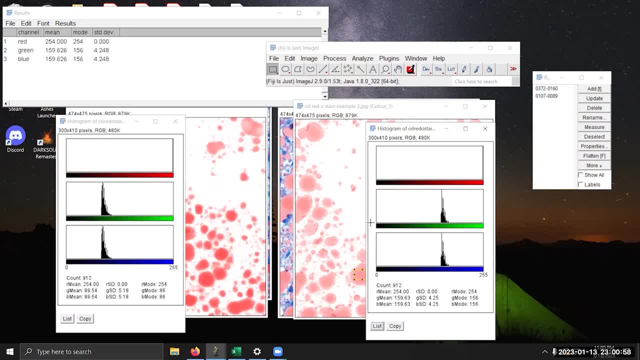 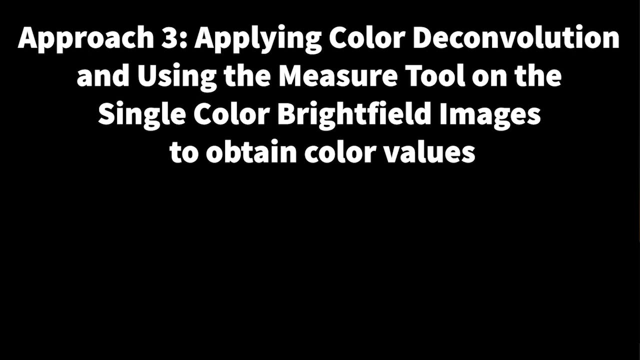 And indeed I believe it does. So we can try a different tool instead. We can just use the simple measure tool. So let me go ahead and set that up real quick. Approach 3. Applying color deconvolution And using the measure tool on the single color brightfield images to obtain color values. 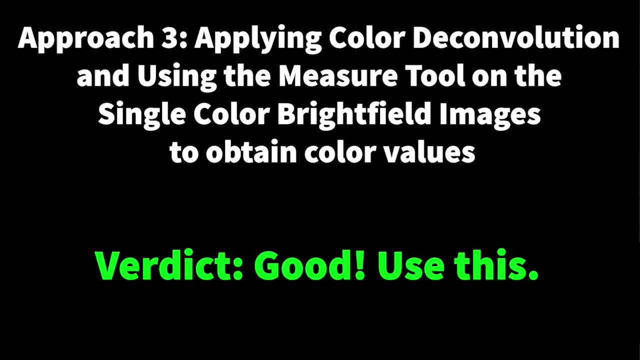 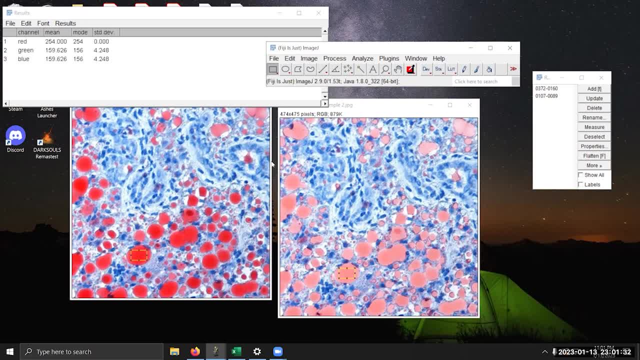 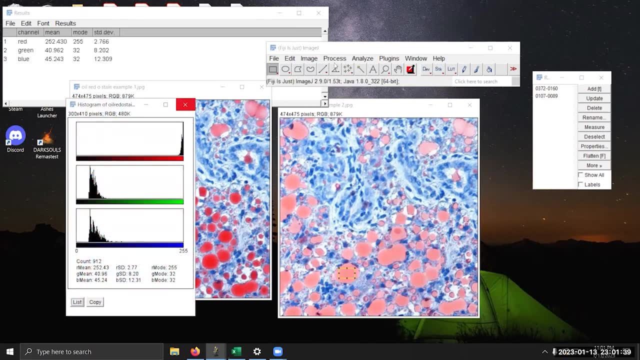 My verdict: Good, Use this. The setup is the same as the last approach. We will apply color deconvolution to these multicolor images in the same way we did before. So color histogram, Sorry. Color deconvolution Image. color deconvolution. 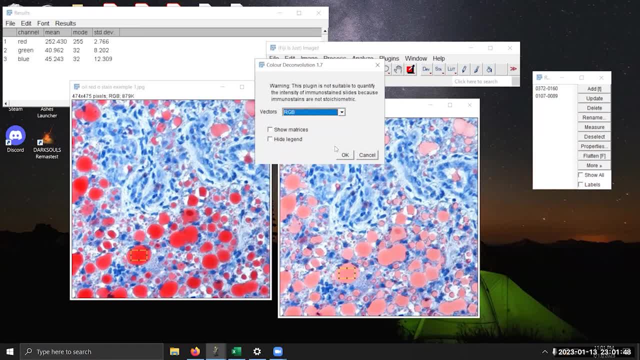 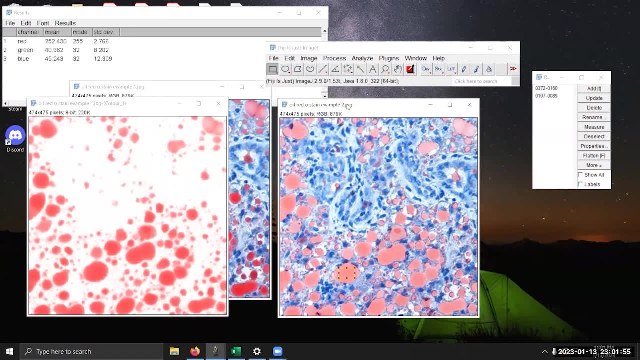 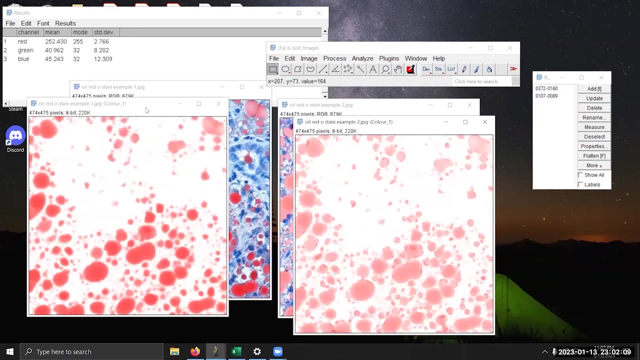 Select RGB. in this specific case, We can get rid of the green and blue channels for now, And we will do the same thing with the faded stain Click, And now we just have the red left behind. We will draw our selection boxes using the ROI manager again. 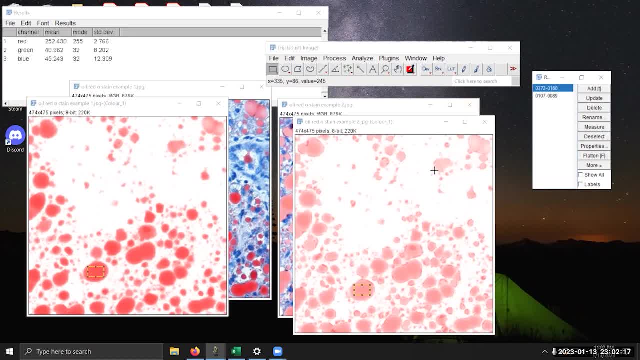 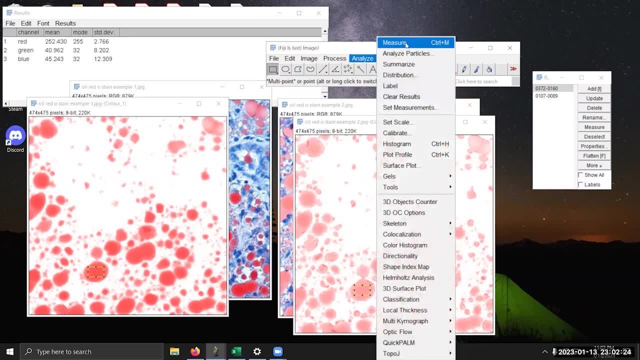 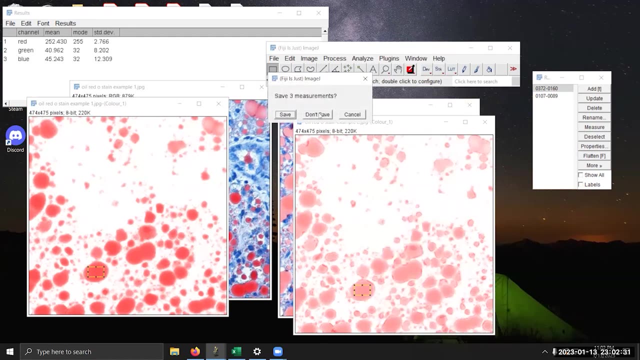 Okay, Now click on the first red window And go to analyze measure. You will notice that the shortcut is also control M if you want to do this more quickly. So I will hit analyze measure. We are going to click don't save. 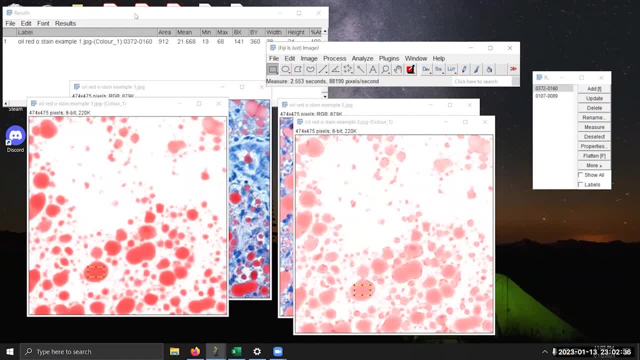 To get rid of the previous stuff, And now we have our first entry. We have a lot of data here. The most important value that we are looking for is the mean value here, And so that is the mean value from 0.. 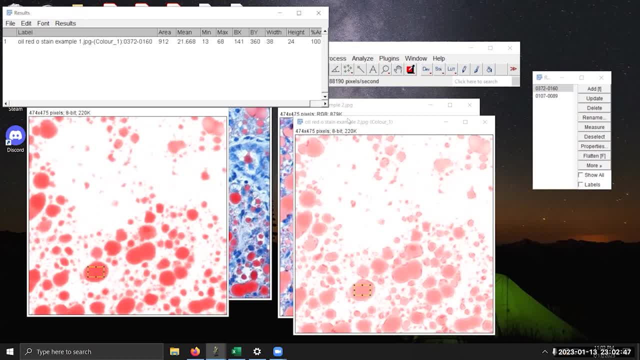 To 255.. Then we click on the second image And we use the measure function for that as well. We will then look at the results window. You will notice that the mean intensity for the stronger or normal stain is actually less. This may seem counterintuitive. 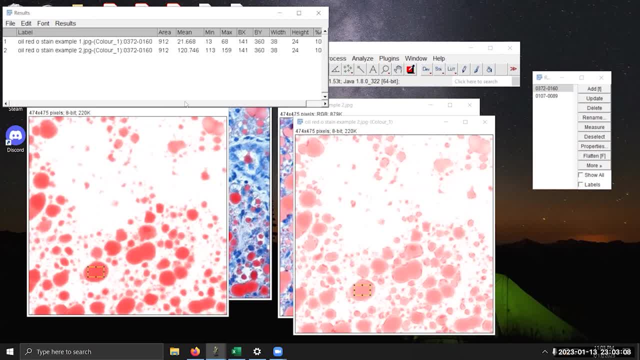 But remember, in bright field imaging, and especially in these single color 8-bit images, a higher value can mean closer to white. This might seem a bit confusing, considering what we were just looking at before, though What does 0 correspond to then? 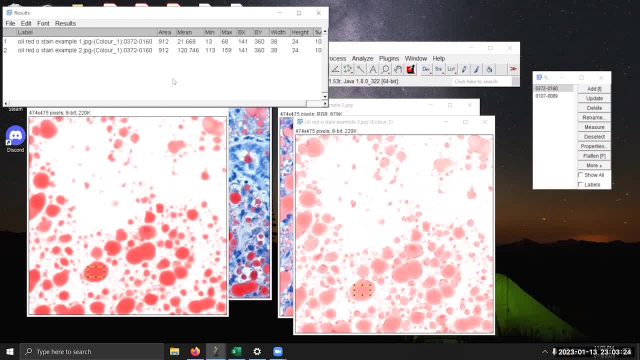 Well, the images that the color deconvolution function produces are 8-bit color images. What this means is that there is the true or pure version of the color that exists at the value of 0. And then values going up toward 255 become increasingly white. 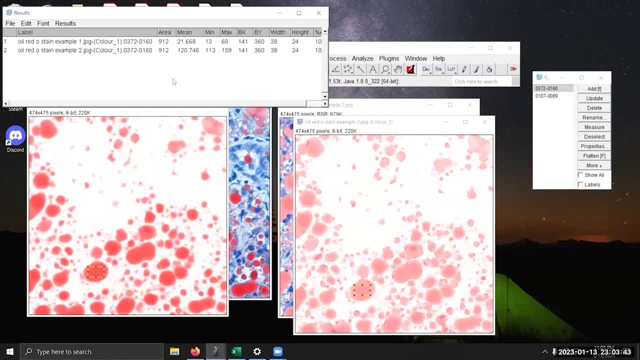 In this case, there is no black color. Black is replaced by the specific color of interest, Again red in this case. Referring again to the results window, these are isolated values you can use to determine the intensity of your particular stain in one color at a time. 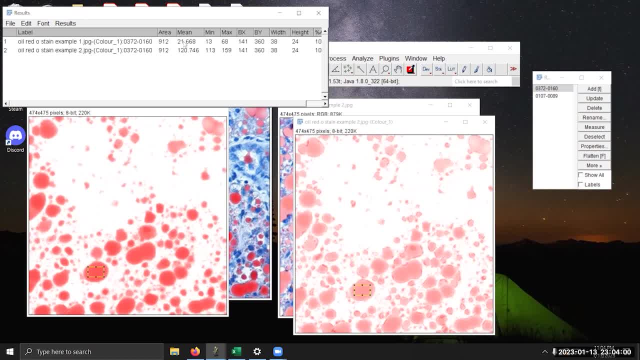 So the values we will be comparing in this case are 21 and 120.. The rest of the data just has to do with either the minimum or maximum color values within the selection box or the dimensions of the selection box that you have acquired. 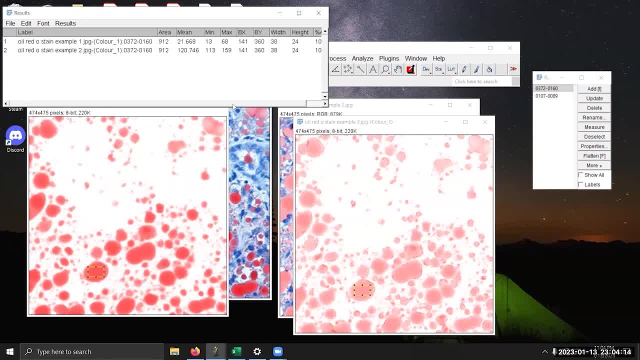 So that approach seemed to work pretty well. The numbers seem pretty distinct. That matches up with how visually distinct they are, And the approach seems to work in a relatively straightforward manner. Hence why I recommended this approach, number 3.. However, some might argue that color deconvolution makes some calculations and estimates in order to split up the colors into separate images. 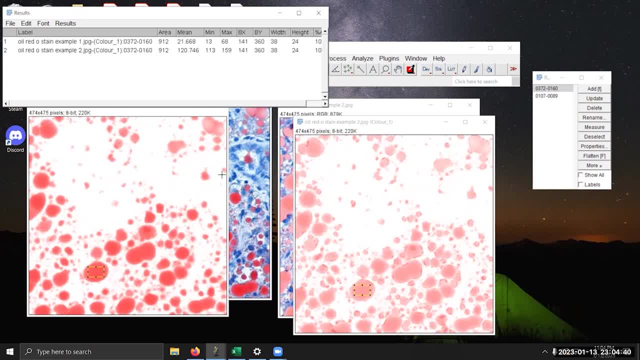 And thus it may have some errors in how it creates those single colors. There is another option for isolating color channels that is more often used on images acquired via fluorescence microscopy. That is the split channels function. However, let me show you why that doesn't work. 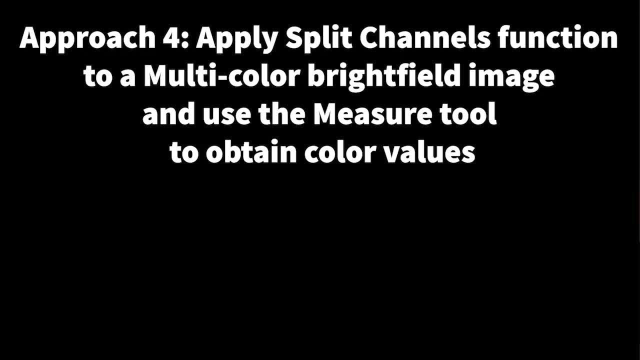 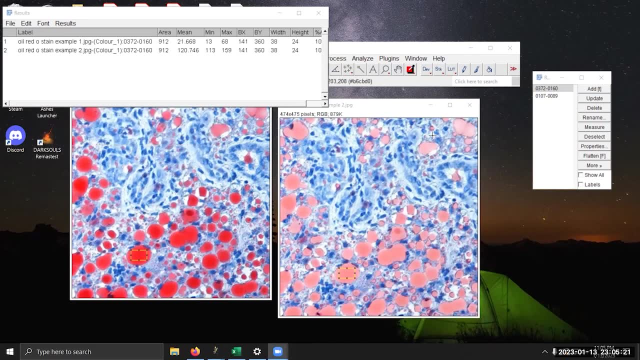 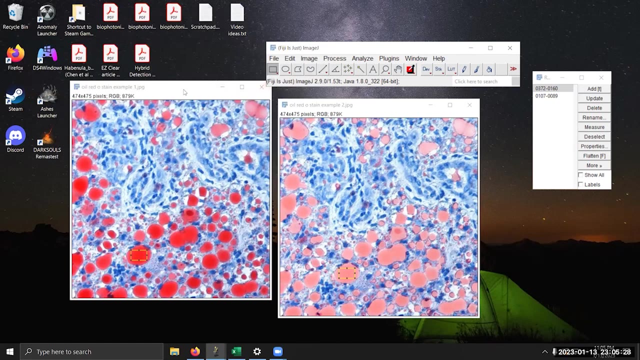 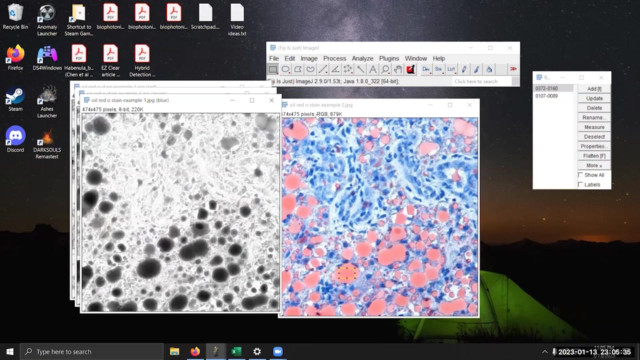 Approach 4.. Apply split channels function to a multicolor bright field image And use the measure tool to obtain color values. Verdict Works, but not ideal. Go to your original multicolor images For each image. go to Image Color Split Channels. 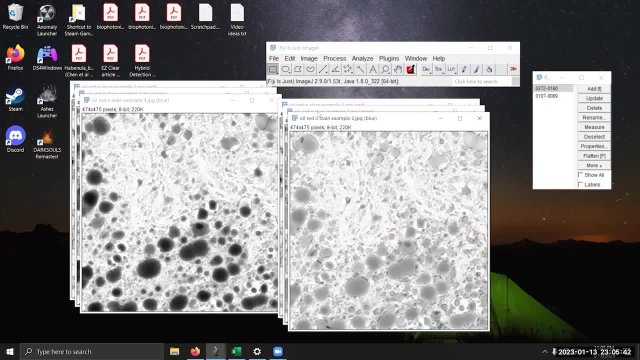 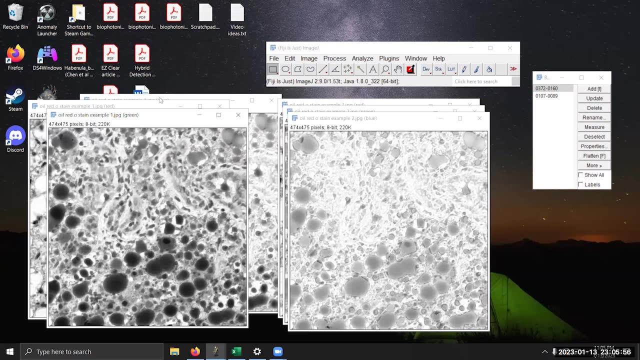 Each of the resulting images are in 8-bit grayscale mode. They are also helpfully titled with their primary color: Red, green and blue. So we see red, green and blue. Example 1 corresponds to the normal stain. 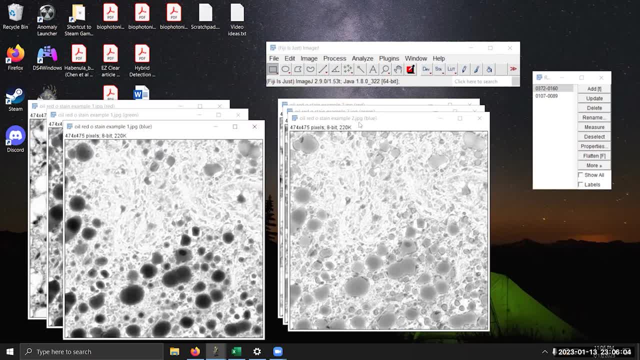 Example 2 corresponds to the faded stain in this particular case. But now that I have the color channels as images, I'm going to show you a glaring issue with that. The issue here that you should note is that there's actually little difference between the red channels for the normal and faded stains. 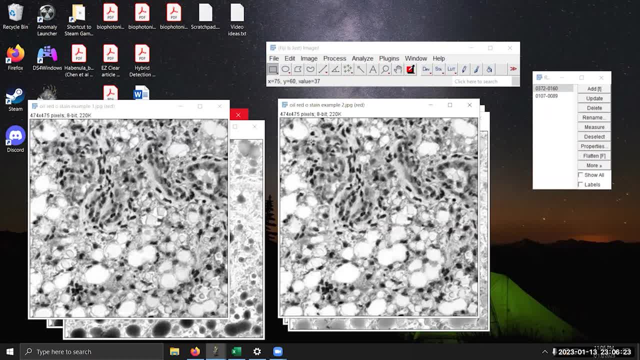 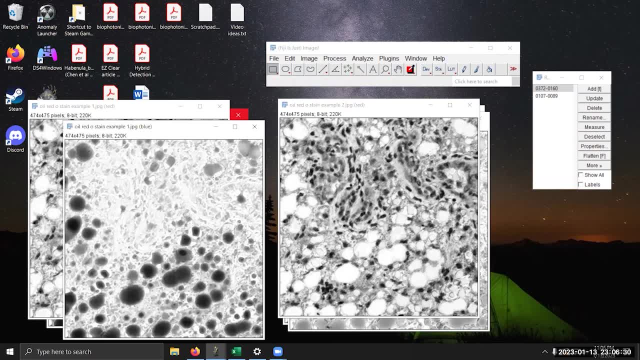 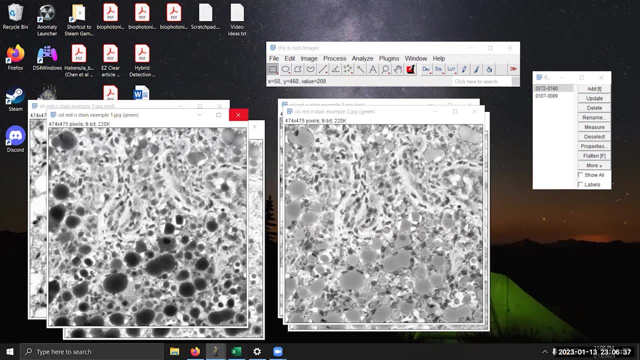 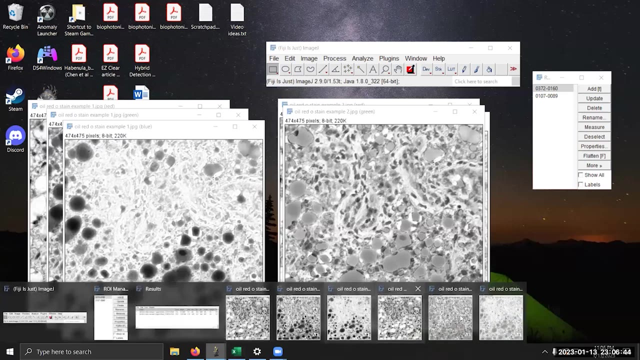 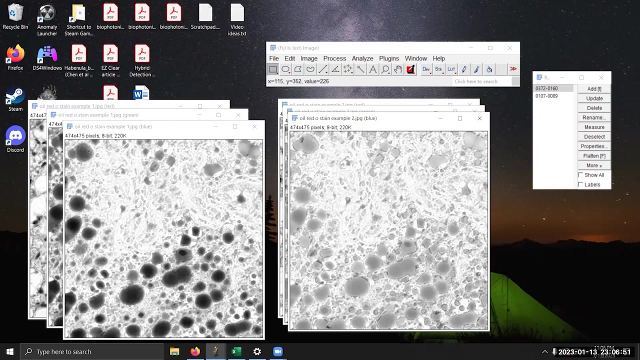 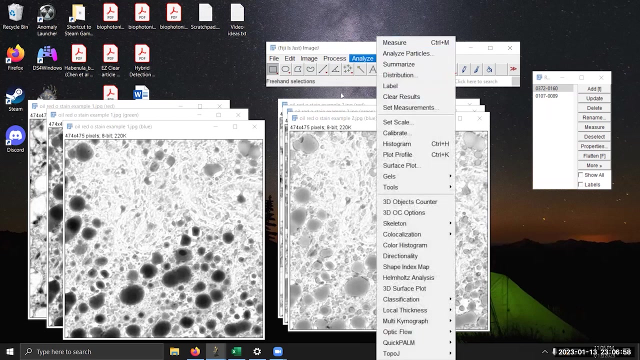 Instead the differences lie again with the blue and green channels. Here we have green, compared They look very different where the blobs are. And then we compare the two blues, And again they look very different where the blobs are. Now you could still measure the differences in those blue and green channels in those particular locations just using the analyze measure tool. 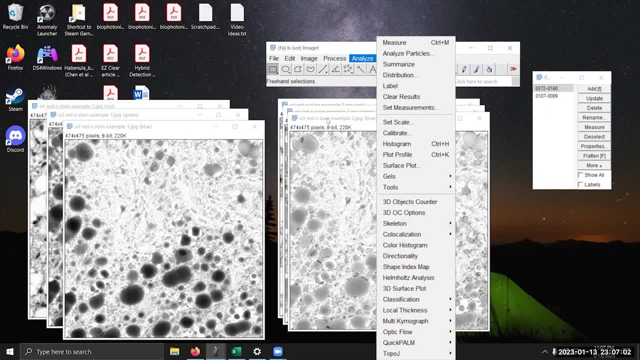 But again it does seem counterintuitive. In general, though, I only find the split channel function to be useful for multi-channel fluorescence images rather than bright field images. But again it does seem counterintuitive. In general, though, I only find the split channel function to be useful for multi-channel fluorescence images rather than bright field images. 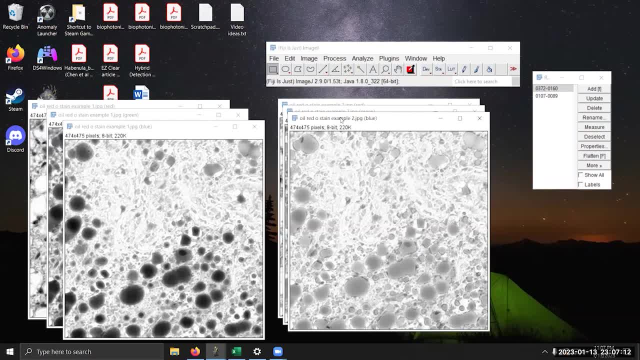 So I would say this approach number 4 doesn't seem to be all that helpful, And we'll see that. when I did go through the trouble of doing it, as I'll show you the data, the results end up coming out being basically identical to approach number 1,. 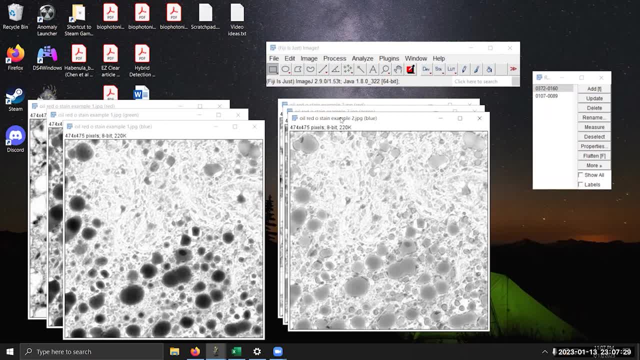 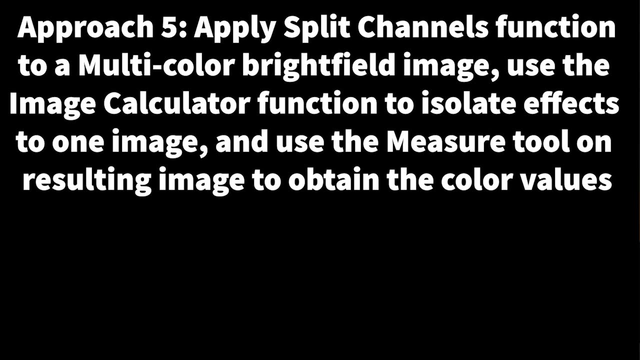 where we didn't have to do any sort of channel splitting in the beginning. But maybe there's still something we can do with those separate channels to get the fading effect into just one image rather than split across two. Approach number 5. Apply split channels function to a multi-color bright field image. 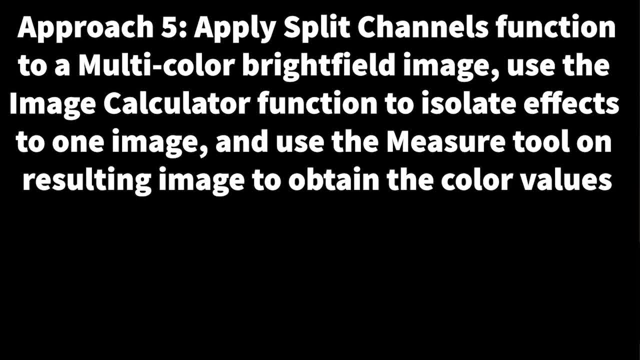 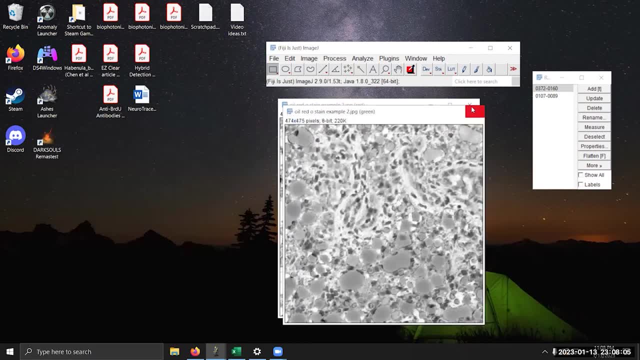 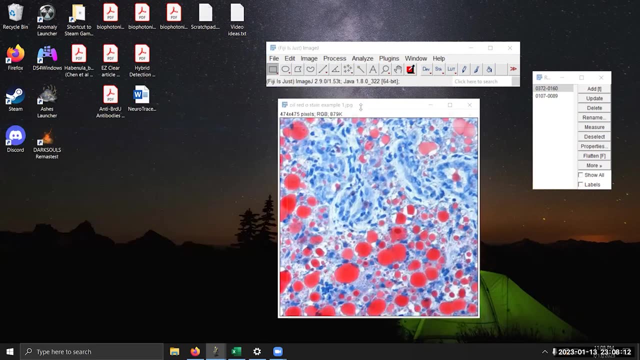 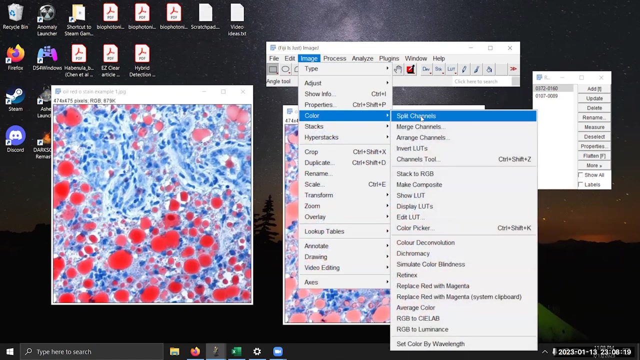 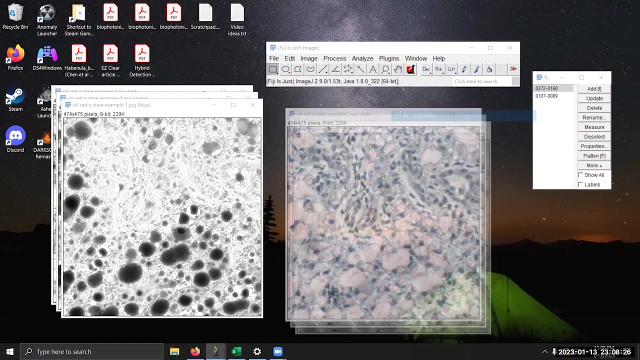 Use the image calculator function to isolate effects to one image and use the measure tool on the resulting image to obtain color values. My verdict: It works, but it's complicated. Let's go back to the original multi-color image. For each multi-color image, we will again go to Image Color Split Channels. 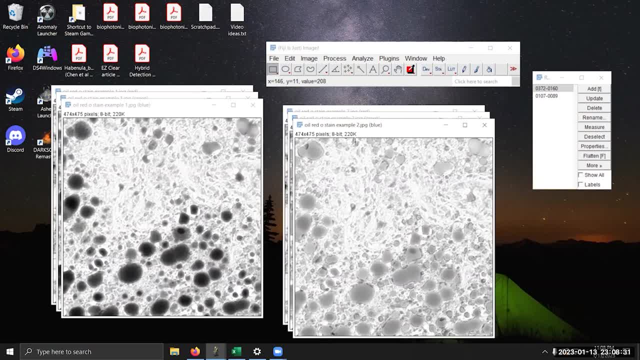 We again get these three 8-bit grayscale mode images of the red, green and blue channels. For the first set of images coming from the normal stain on the left titled Example 1, here we will run them through the image calculator. 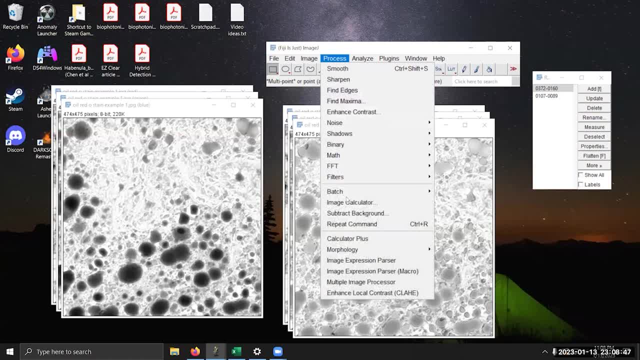 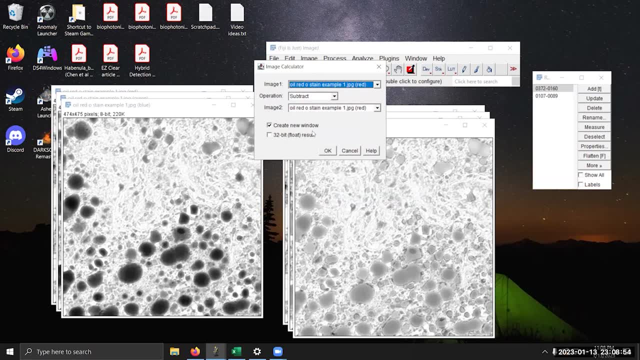 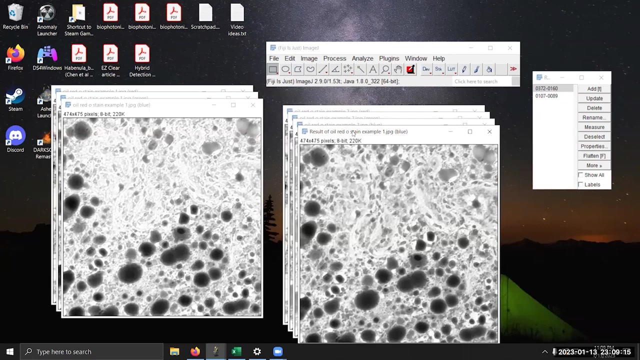 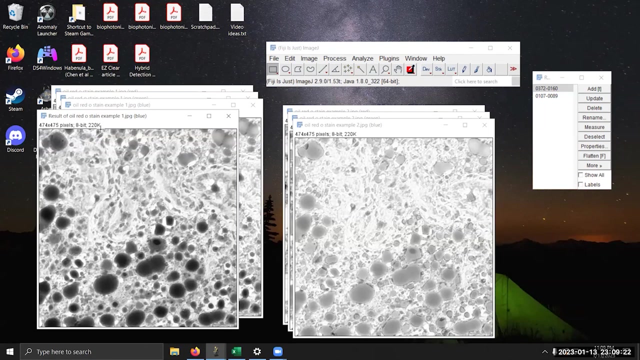 Go to Process Image Calculator. First, select the blue and green channels and select the function Average. This will create a new picture with Result at the beginning of its title And this is the average of the blue and green channels. Despite the ending of it saying blue, this is the average created by that. 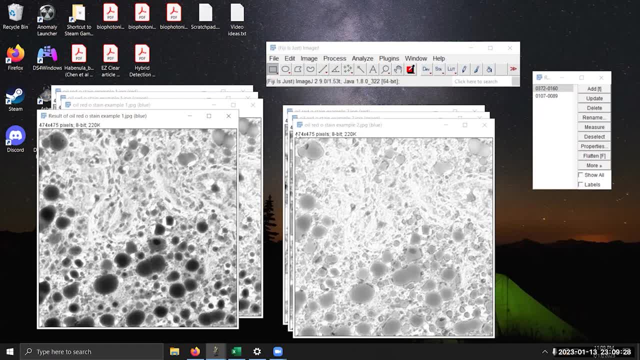 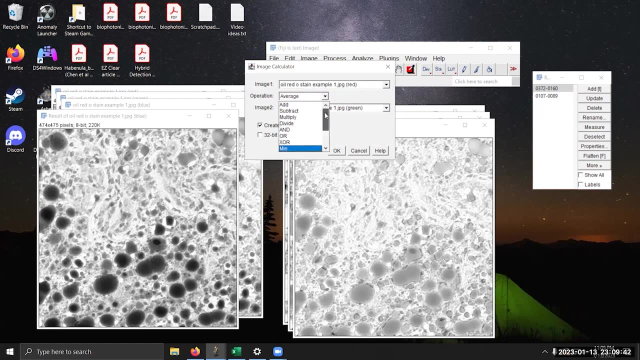 You will then subtract this particular image from the corresponding red channel. So we go back to Process. Go to Process: Image Calculator. Select the red channel in the first box- The operation should be Subtract- And select the result image in the remaining box. 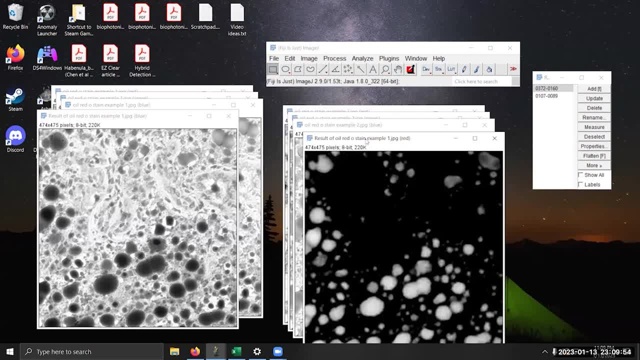 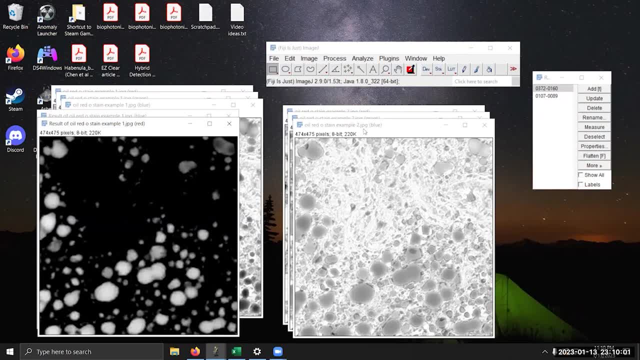 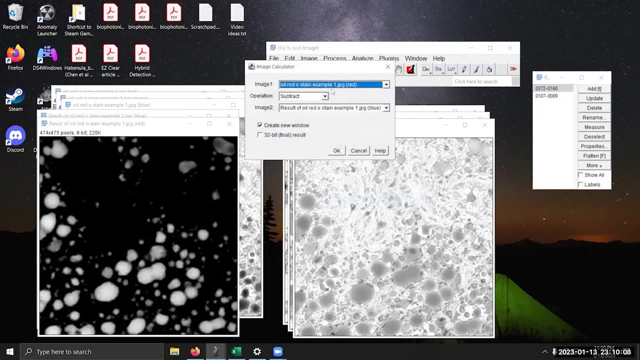 Hit OK. This produces another new image, So we will repeat this process all over again for the second set of images, Example 2. Coming from the faded stain: If we are going to introduce extra colors and changes in color, we use a double click layer. 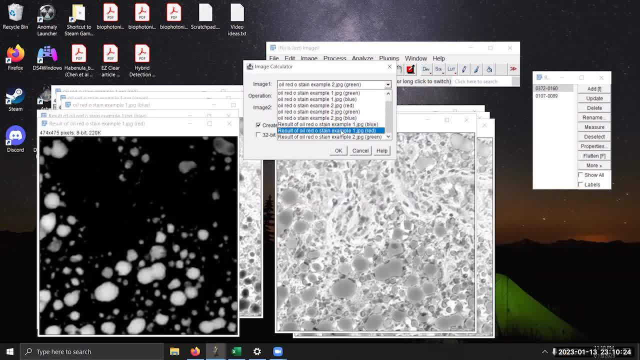 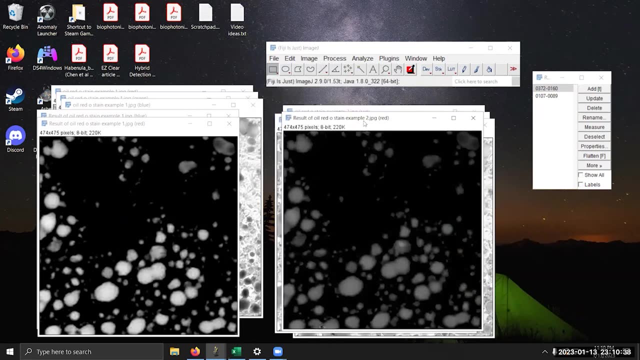 Use the fired black color layer to please. Let's see what changes these changes will have. At this point it is busy and not being shown to the rest of the image. It won't say: the image has the color. Now you can use the measure tool to compare the final products against each other. 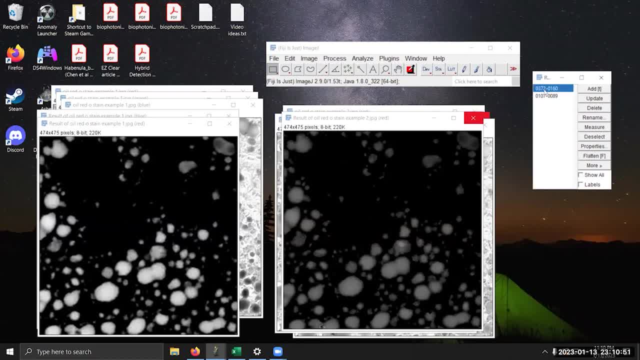 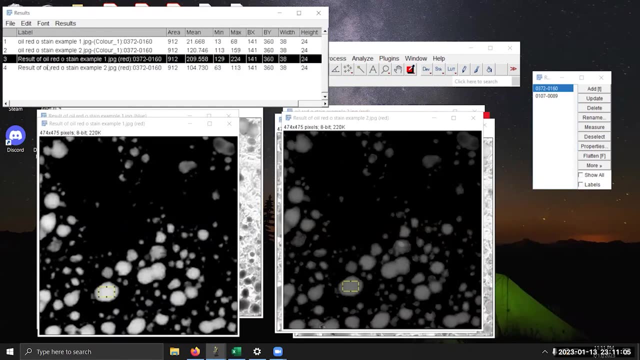 I'm going to use the ROI manager to draw the box in the correct locations again, I'll hit control M to measure first, control M to measure the second and we could pop up the box to take a look. These are the recent two ones I just populated. 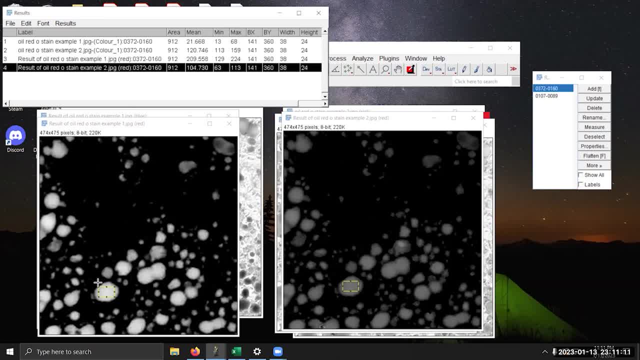 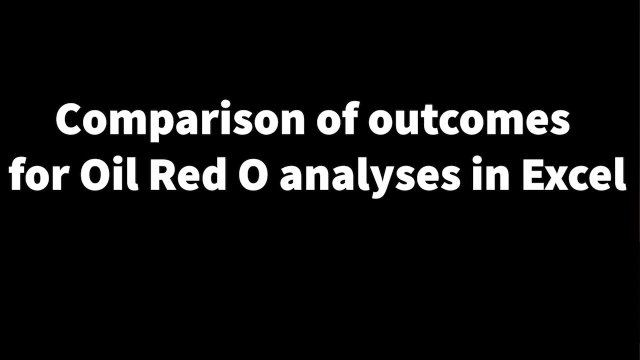 You'll see the numbers 209 and 104.. 209 corresponds to this one, 104 corresponds to this one. I'll talk about why one number is greater than the other in a little bit. when we talk about the data, Let's look back at our values that we attained from this process. 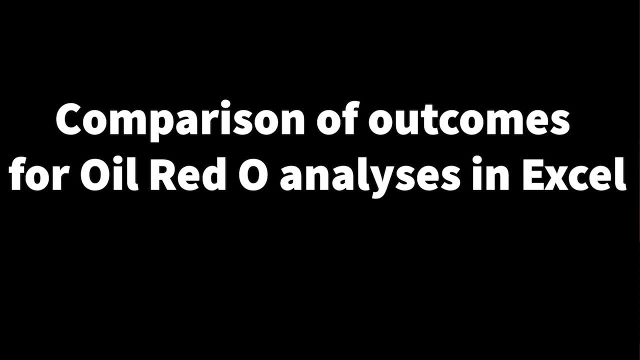 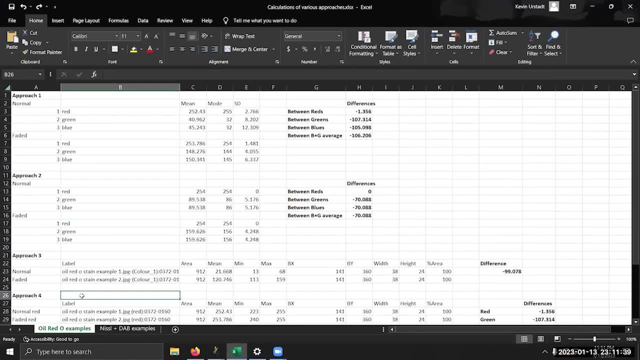 I copy pasted these values in Excel in advance so I could compare the calculations on screen. Let's take a look For approach number one, where we used color histogram on the original multicolor images. we can see a minor difference in red between the two images. 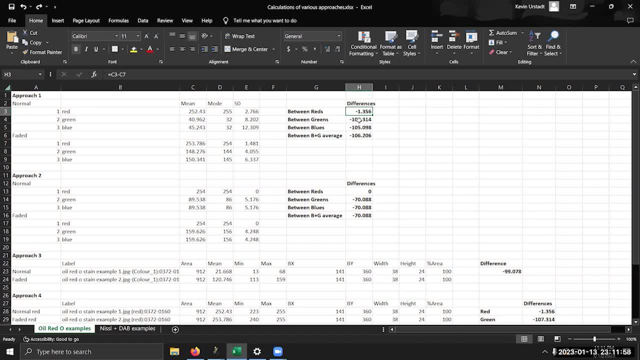 The normal and faded stains, And we see also very similar magnitudes of differences between the greens of the two stains and the blues of the two stains. Now, these may be more appropriate. I also determined the averages of the differences between the blue and green stains. 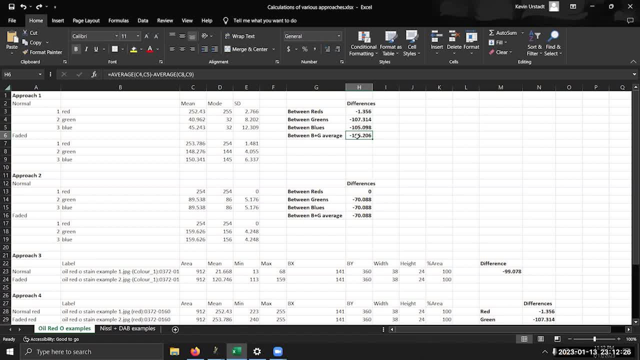 So I basically took the numbers here and here And then figured out their average. And figuring out this average may be more appropriate for anybody working with colors that are not exactly red or blue or green, and may instead be things like cyan, purple or yellow. 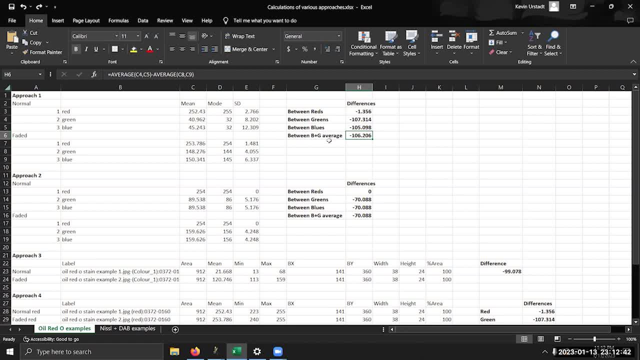 Okay. So if we're looking at the color difference in the colors other than red, it's about a hundred shades difference out of 255 possible shades. magnitude difference For approach two: Okay, So if we had applied color deconvolution and use color histogram tool on just the red channel? 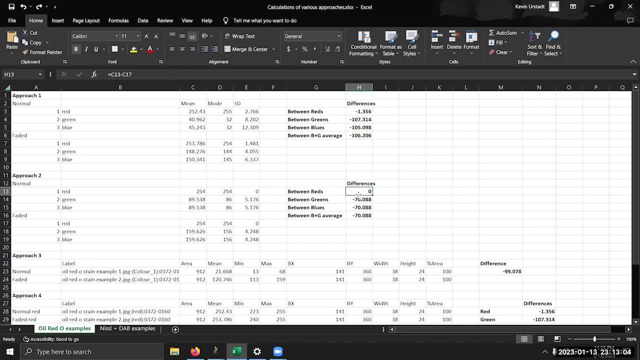 we see, the difference between reds is zero, The difference between blues and greens is identical. So when you get the average it's going to be again identical, And yet these values are noticeably different from the approach and one's results. So I don't necessarily trust these values to be inappropriate. resin representation. 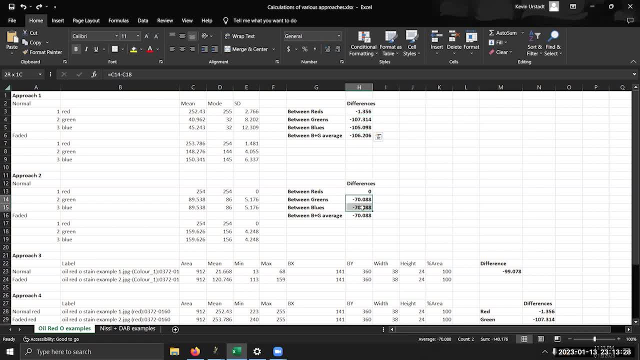 So, rather than getting something closer to a hundred, we see that these are somewhere around 70.. You'll see how the other values aren't really close to 70, which is why I don't really trust trust approach, one approach to to give us accurate data for approach three, in which. 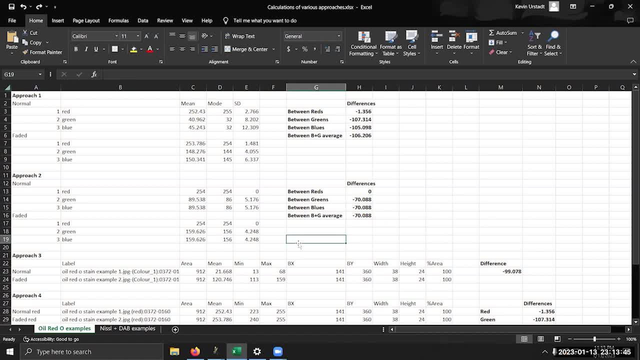 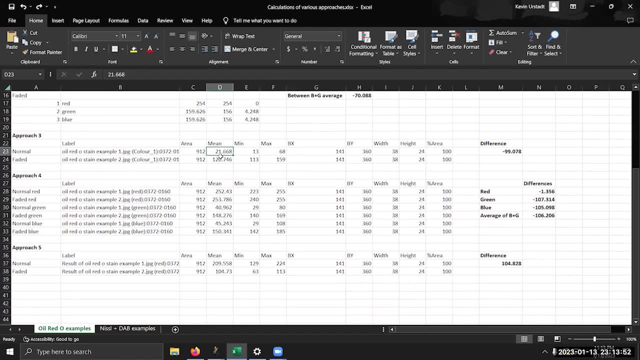 we did use the color deconvolution And then we used the simple measure tool. The simpler intensity difference between the stains is 99. So we figured out the difference between these two And we get the number of Okay. So we have a value of minus 99.. 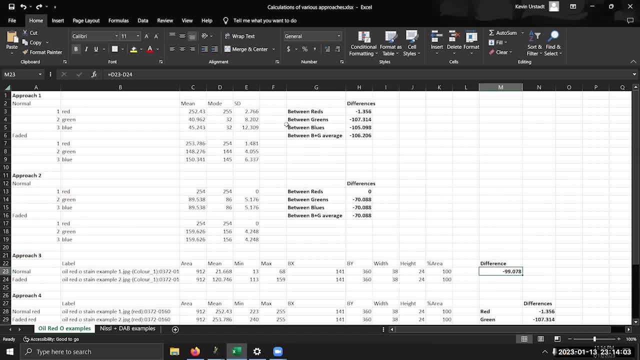 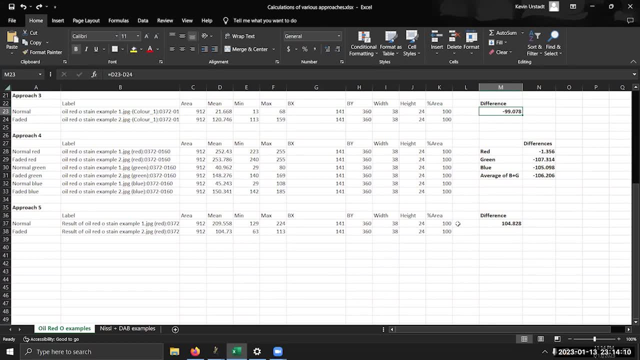 This value is similar enough to the results from number one, approach one that I generally trust it. for approach number four, in which we applied the split channels function to the original images And then I, off recording, measured the intensity for each resulting channel, You'll notice that the results are identical to those of approach one. 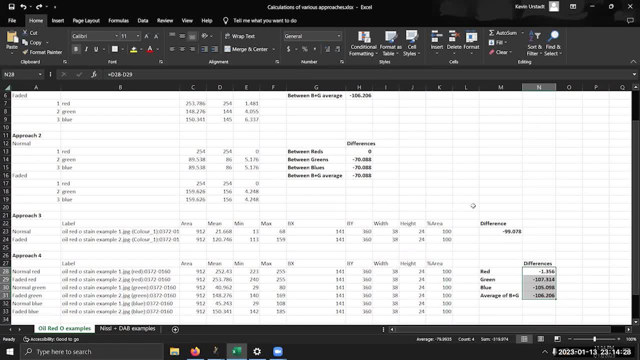 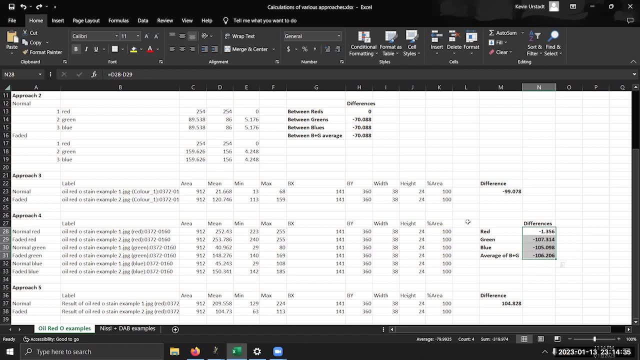 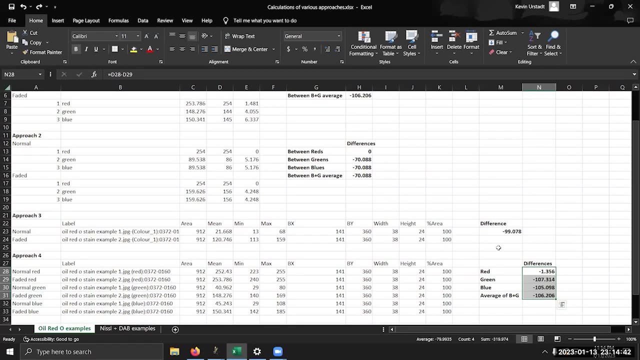 And that is because the color histogram tool measures the raw intensities of red, green and blue after isolating them as channels. So basically, doing approach four is a very complicated and convoluted way to get the same data that you would get with approach one. 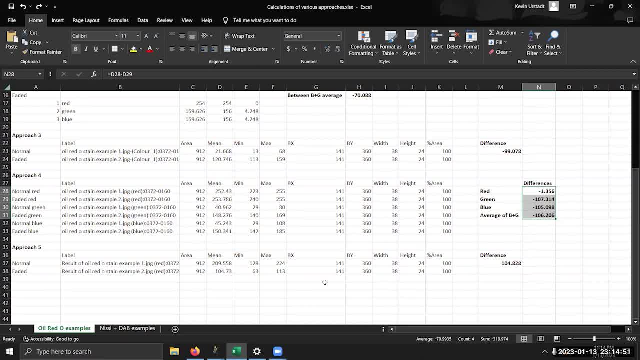 And then we have approach five, in which we did the split channels function on the original multicolor images And subtracted the blue, the average. we subtracted the average of the blue and green values from the red channel and applied the measure tool. 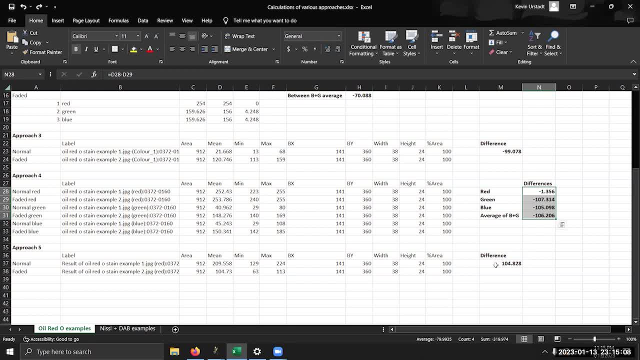 And we get another value that's relatively close to the other, approaches 104.. So somewhere around a little over 100 in magnitude, or close to it. But why is this number not negative like the others? Well, the image subtraction process actually inverted the color range, making it go positive. 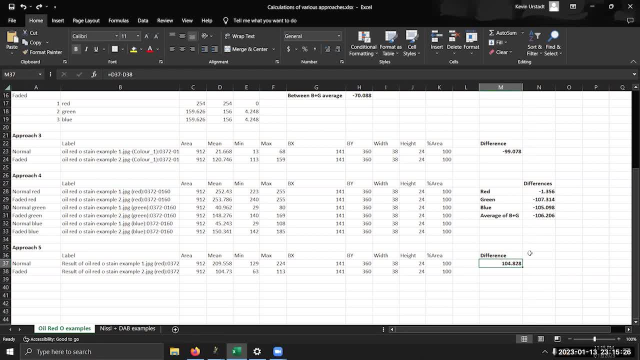 rather than negative. Regardless, the absolute magnitude is probably the more interesting number that you're caring about, much less the sign. All of the above considered, which approach should you use If your stain can easily be separated into red, green and blue? I think that approach. 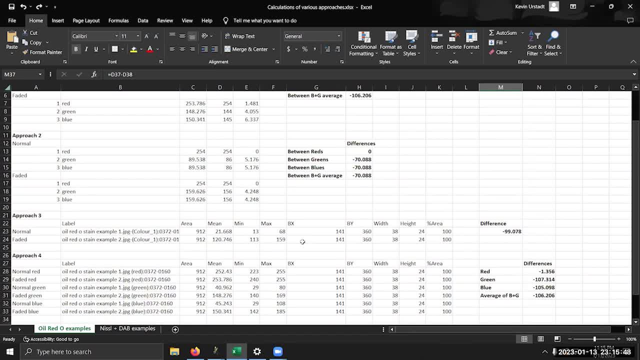 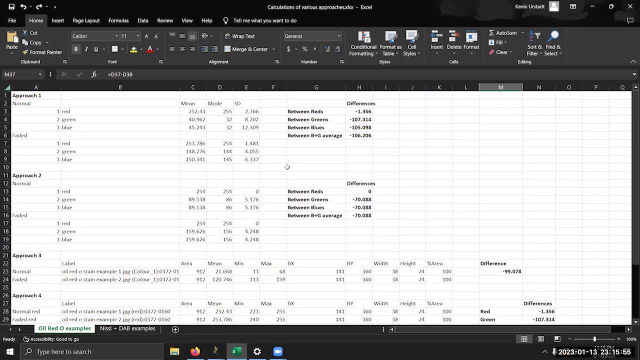 number three or potentially approach number five make the most sense. You could still use approaches one and four, but you'd have to average the effects of the channels that are counter-intuitively not the color that you're interested in. But what if your stain is not an easy red, green, blue split? 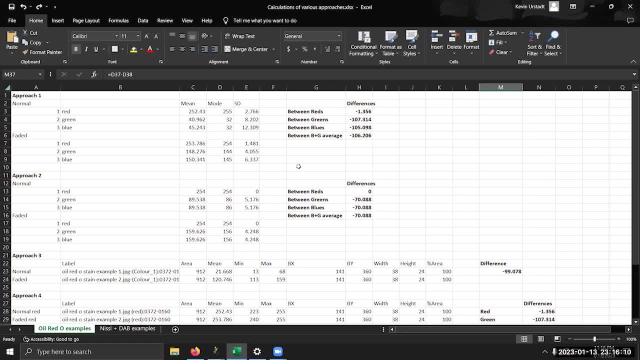 Let's look at another example briefly. I found an image online that used a combination of NISL staining and DAB staining on brain tissue. The NISL stain, although not always, can sometimes take on a purple color, depending how it is used. 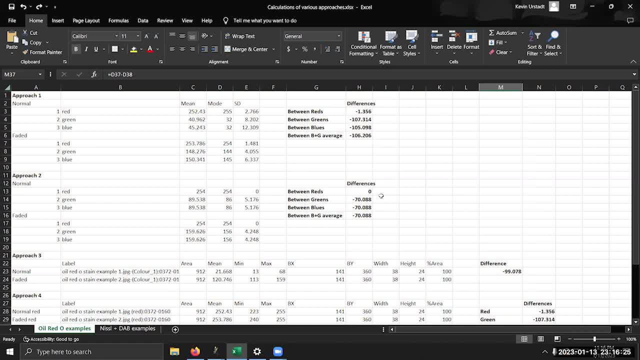 And the DAB stain is typically an orange And the DAB stain is typically an orange And the DAB stain is typically an orange And the DAB stain is typically an amber-brown color. These are not strictly red, green or blue. 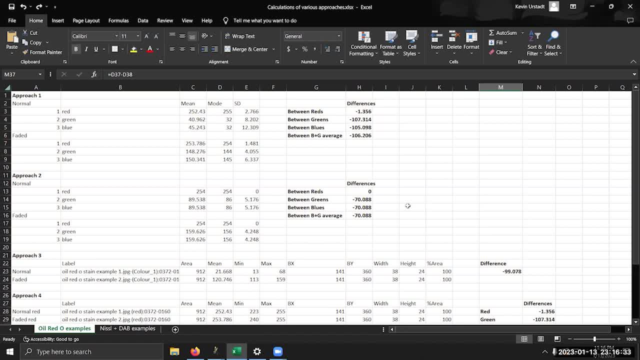 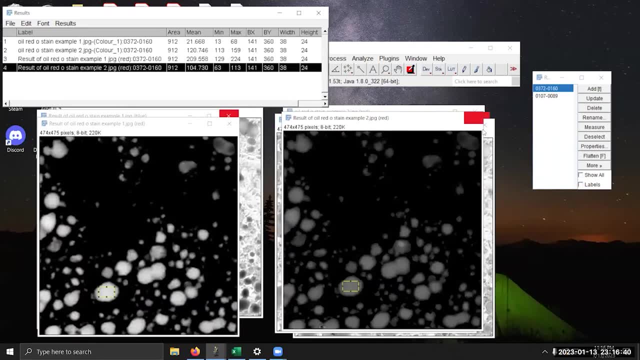 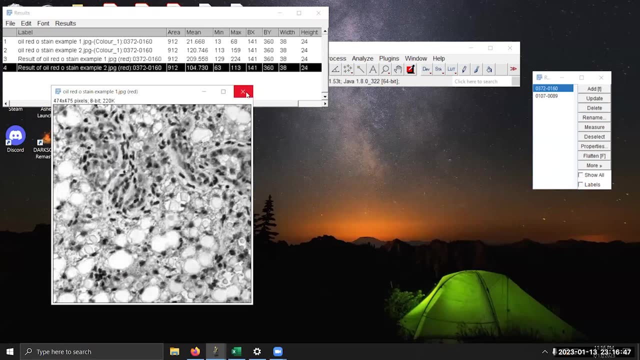 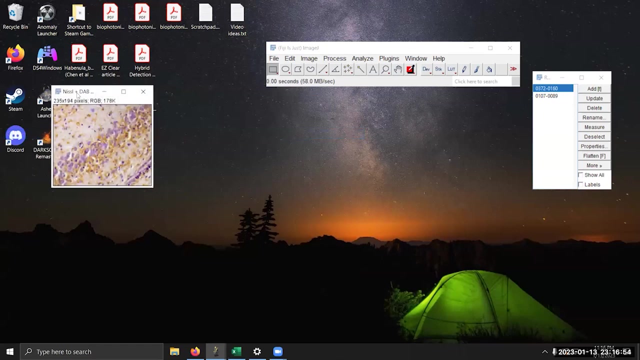 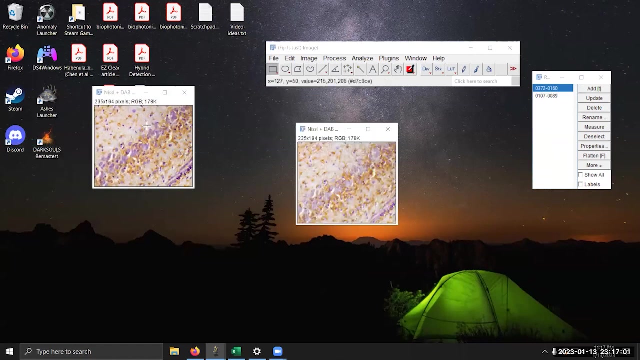 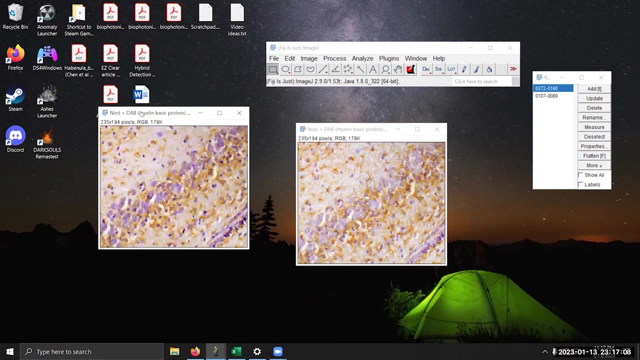 They are colors that are in between these primary constituents. Let's set up for that. Let's set up for that. What you should be able to notice between these two images is that the image on the left has a darker purple color than the image on the right. 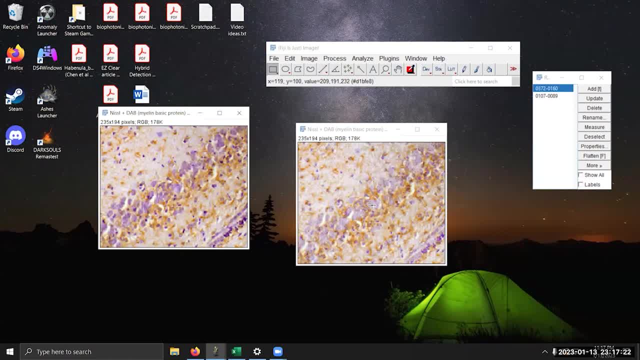 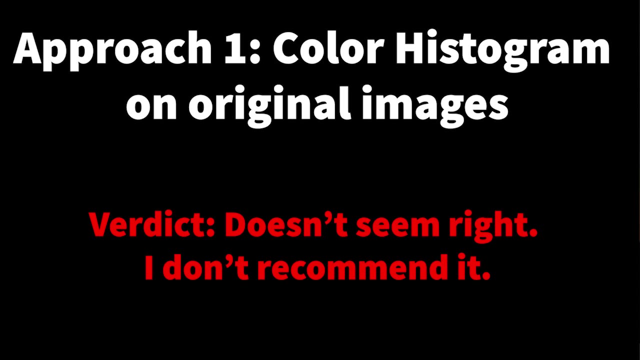 Again, using the GIMP program, I artificially faded the purple color that corresponds to the NISL staining. We can do approach one again simply enough. Approach one on complex non-RGB stains. My verdict Doesn't seem right. I don't recommend it. 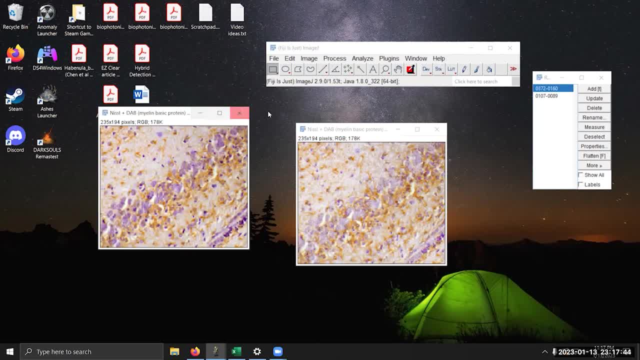 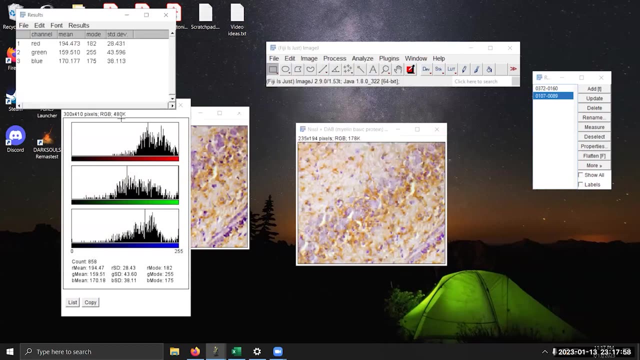 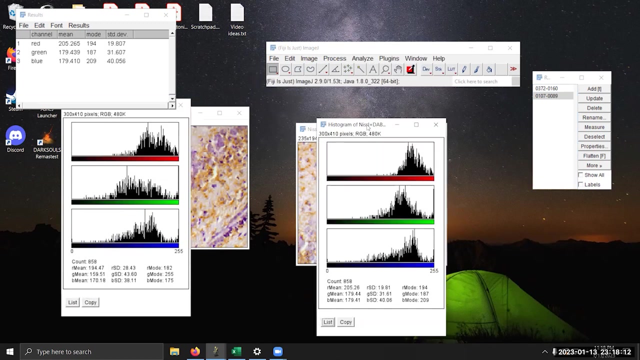 To show you why it doesn't work so well, first select an area of interest in your first image. Use the Color Histogram tool. Analyze Color Histogram Here, Copy the values that it gives you into Excel and then do the same for the second image. 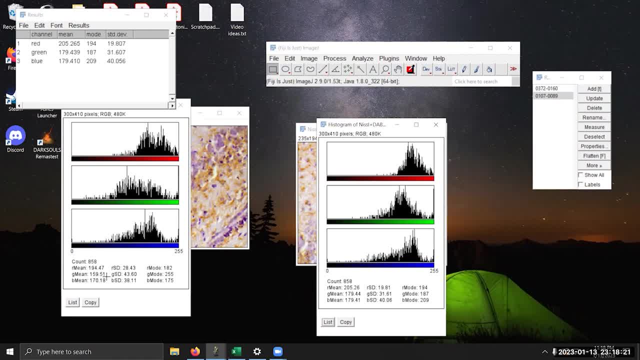 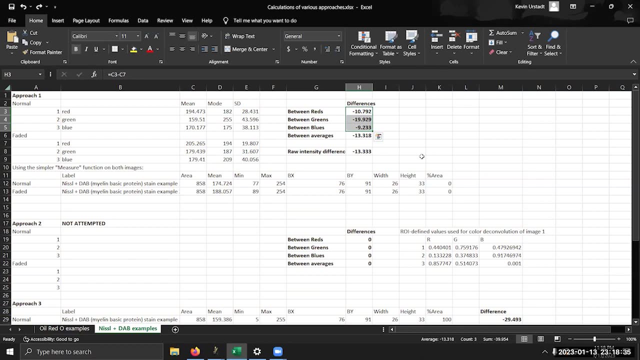 When we see the values presented here in the color histogram windows, we do see that there are slight changes in all three colors, especially when we look at it again in Excel. So that data is up here, the specific differences, And because of this I opted to try to average them together into negative 13 here. 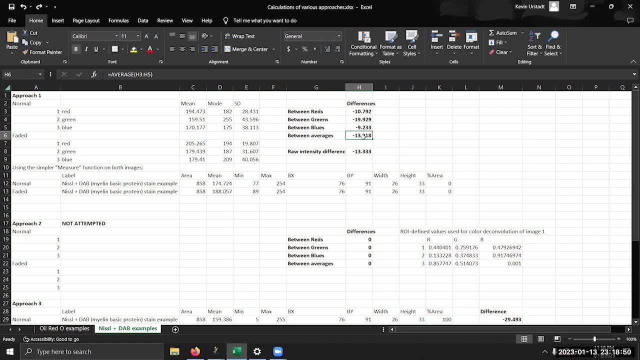 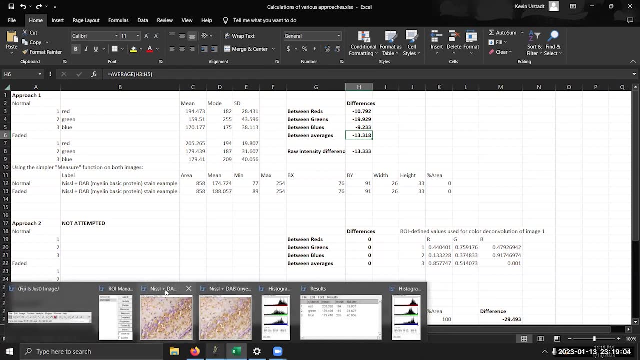 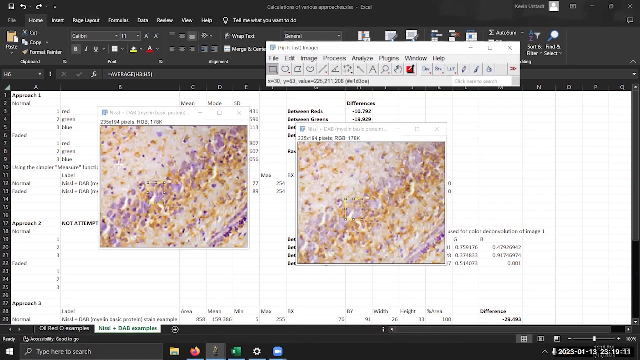 But this average of the three color differences. this is probably the same as if we tried to measure the mean intensity using the measure tool on the original multicolor images. So to check that quickly, take those two same images with their selections and use the measure function on both. 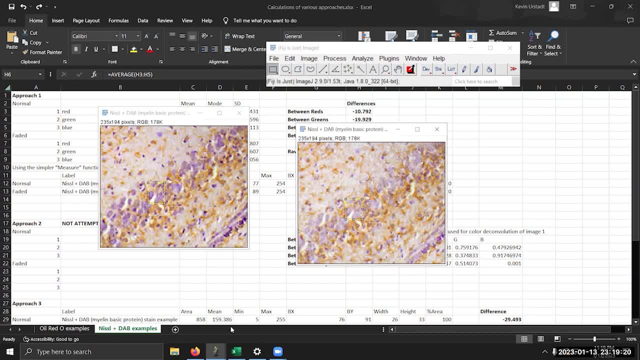 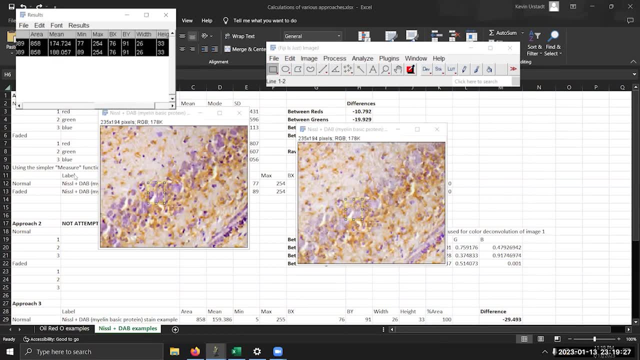 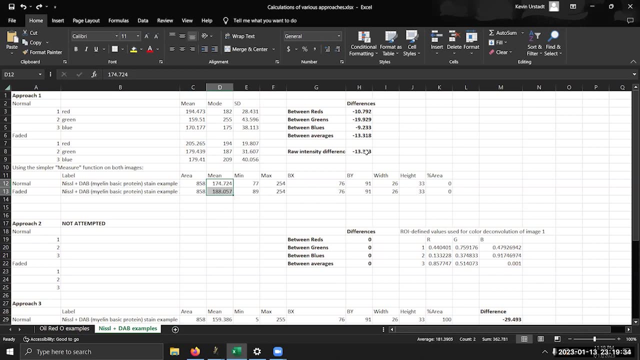 I then copy pasted these values into here- and in particular we are focused here on these mean values- and we again get the result of roughly minus 13.. We can see that after plugging it into excel that the value is nearly the same, meaning that we didn't necessarily need to use a color histogram. 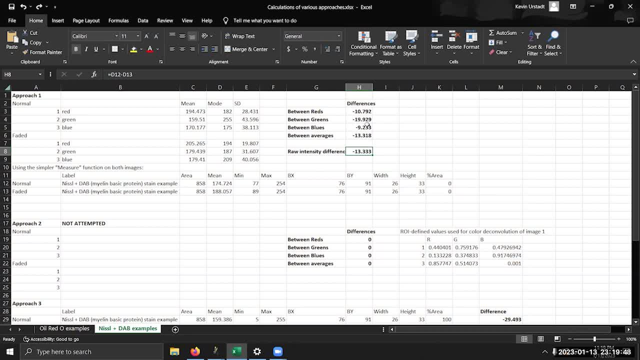 If we just want to figure out what the average Intensity difference was, so that doesn't really tell us much about coloration at that point, Based on the issues that we saw with approach to before, i'm going to skip approach to for this specific set of images. approach to on complex non-rgb stains: verdict: not recommended. 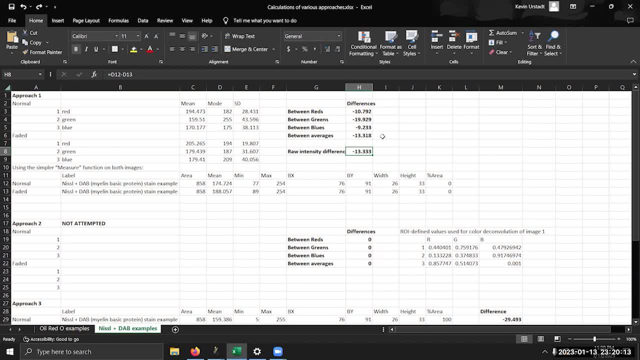 Now applying approach 3 instead gets a bit tricky by, I believe, approach This approach is still the most effective option. If there is not already a setting for your type of stain in the color deconvolution menu, you will have to generate your own setting. 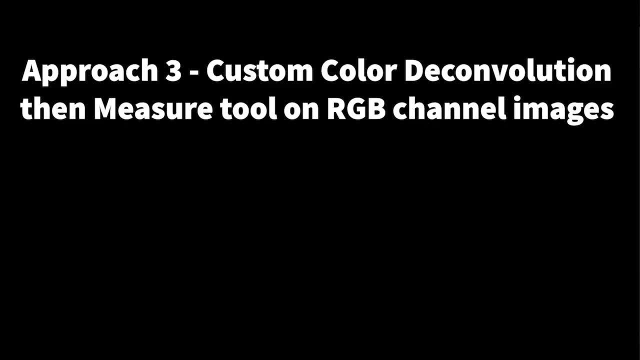 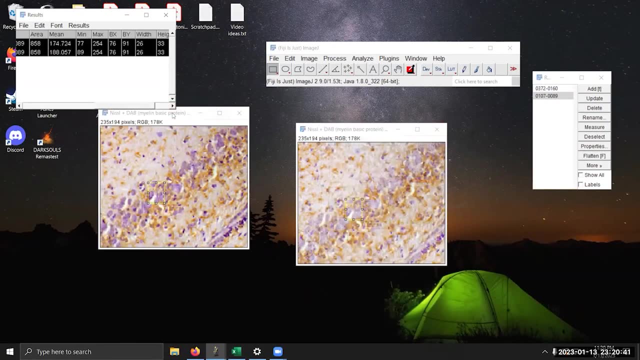 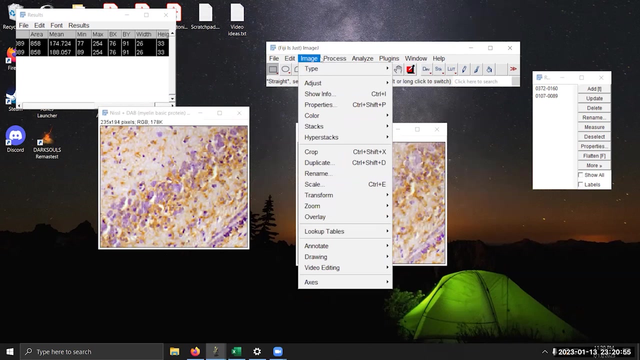 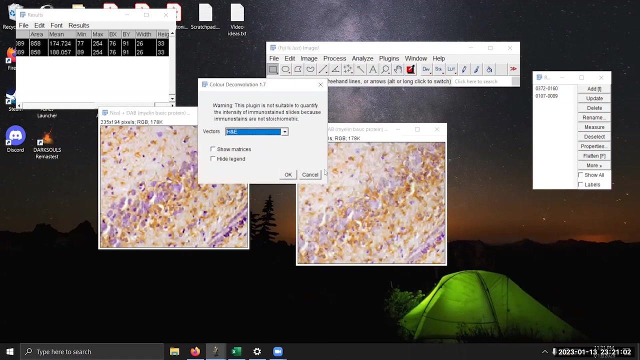 So let me show you how to do that. approach 3 on complex non-rgb stains verdict. Use this: Take your bright field image stain and make sure nothing is selected in the image. Go to the color deconvolution tool. Let me make sure the first image is selected. 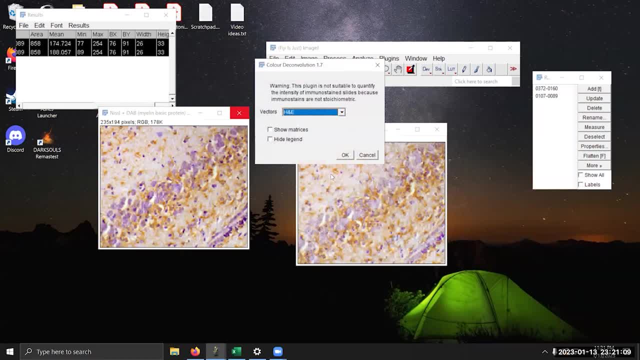 Okay, image color deconvolution. Select the from Roi setting towards the bottom. This setting will ask you to decide on the 3 main colors to split your image into, Even if there are only 2 main colors that you care about. 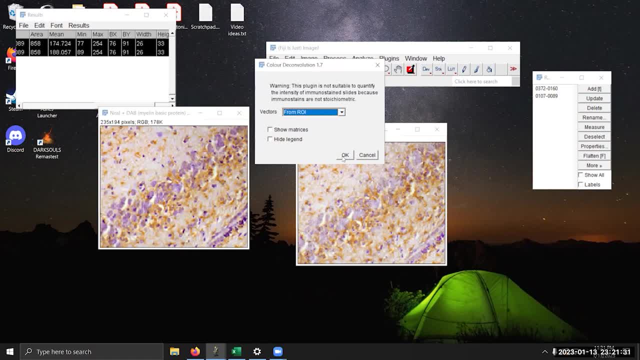 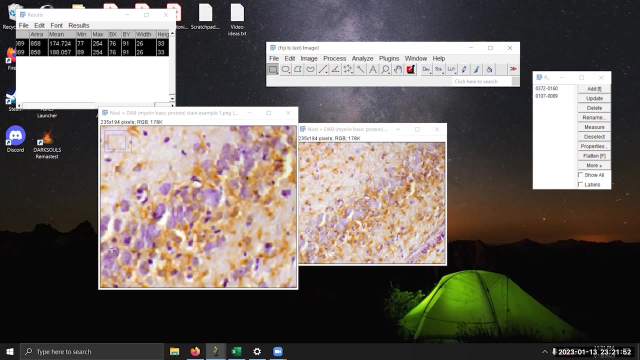 You can still use this tool. When you do the from Roi option, a dialog box will appear. click Okay and then draw a selection around the most typical Or ideal stain for that color. for this nistle stain, I will draw a box around a cluster of purple blobs. 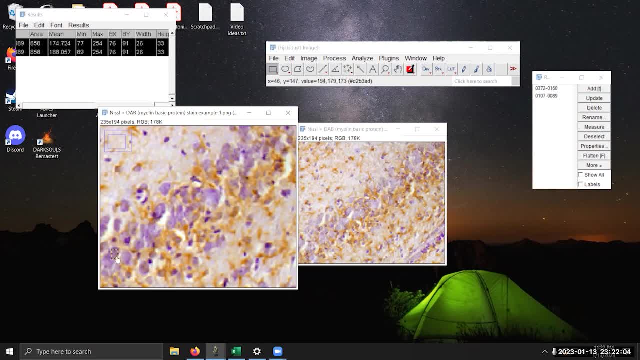 Or even around one singular purple blob, And then a selection: right click. As a side note, I'm unsure what the other option will be for Mac users. instead of right click, It may involve holding the command button and clicking rather than using right click, since that doesn't exist on Macs. 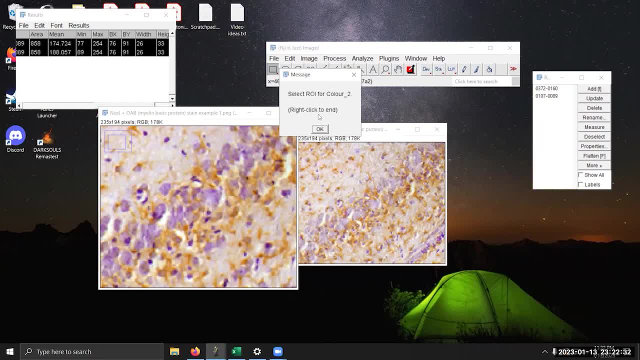 But hopefully your dialog box will tell you specifically what you should be doing instead of right clicking. So after you get this dialog box, click okay And select the other stained element in the picture. for this Dab stain, I'm selecting a cluster of brown blobs with no purple staining in it. 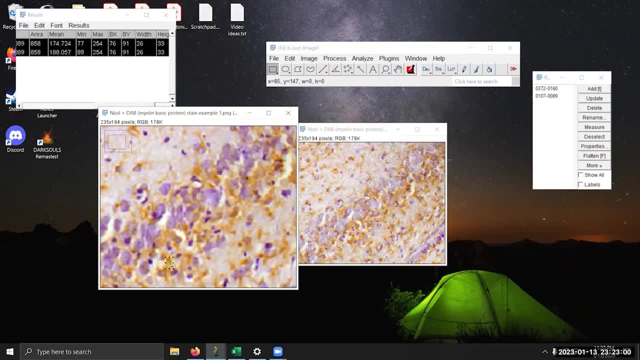 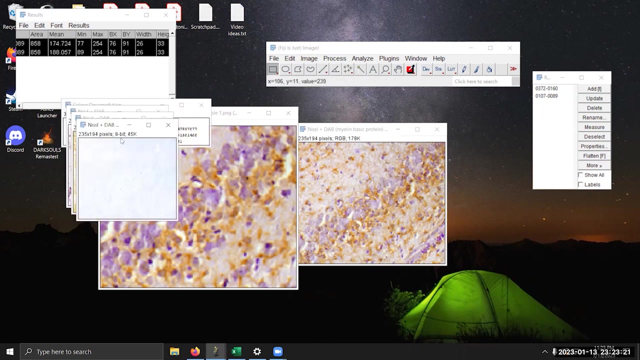 And then right clicking to end the selection. If you don't have a third color stain After hitting okay for this color 3 dialog box, you can just not select anything and right click anywhere on the image. So rather than selecting any sort of thing if we don't have a third color of interest, I just right click here. 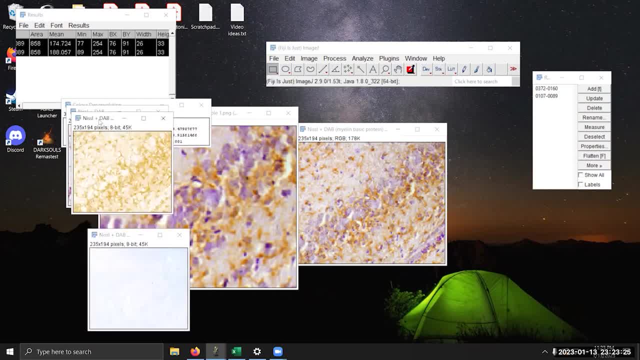 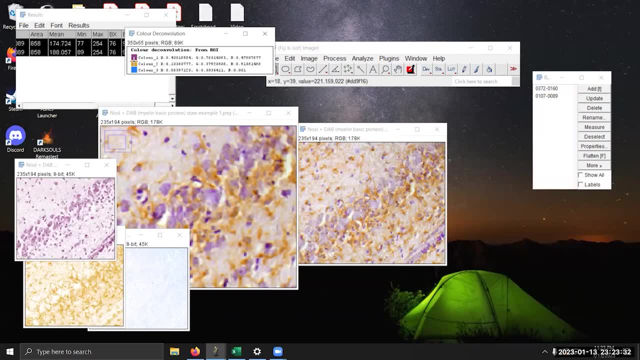 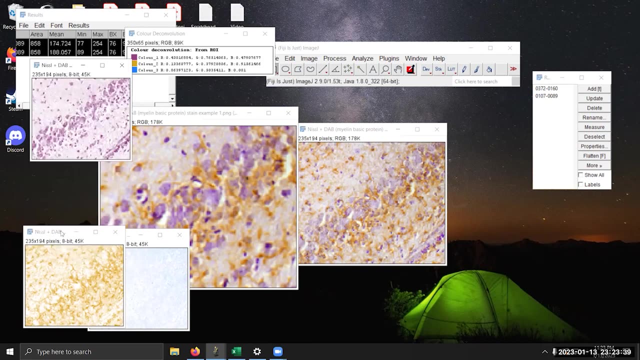 And it automatically pops out the images. So these are the color deconvolutions. You'll notice that it gives you the specific colors that I decided to split. We see purple, We see sort of amber brown And we see blue, And these are appropriately split in these channel images. 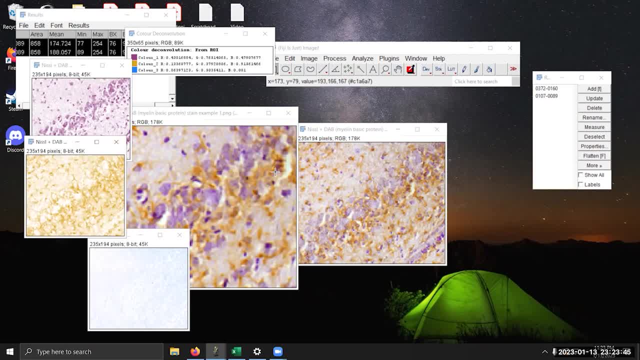 So the tool will do the deconvolution, But more importantly, it will also supply us with the exact color values. we can then save and reuse for later. Although you can't directly copy from here, you can at least manually read out the numbers and copy them into Excel. 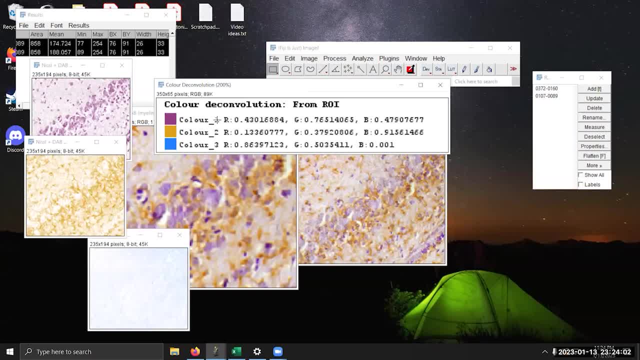 If the font is too small to see, you can magnify this color value window here By using the mouse wheel to scroll up or holding control, and using the mouse wheel, Using the touchpad scroll function or the control plus keys to zoom it in and out. 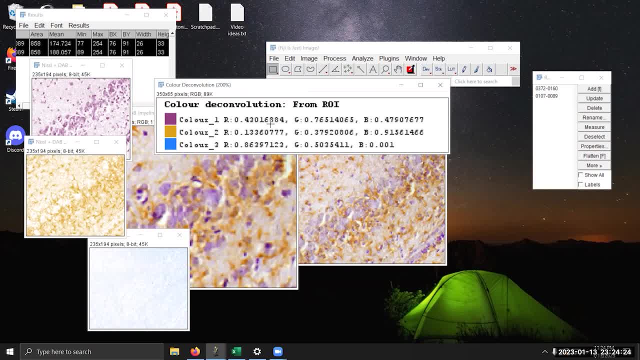 Outside of this recording, I manually copied over the R, G and B values for each of these key colors used in the first image's deconvolution. Although we don't really care about the blue colors values, We still need to keep that in mind. 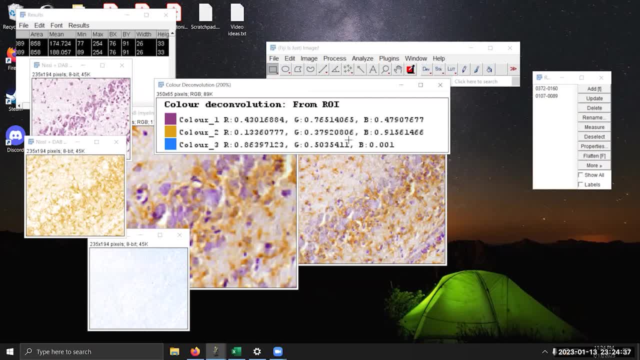 We still need to keep them and use them for when we do the next step, So you'll want to copy down each of these. Purple color consists of this number for red, this number for green and this number for blue. Amber color consists, for this number red, this number green, this number blue. 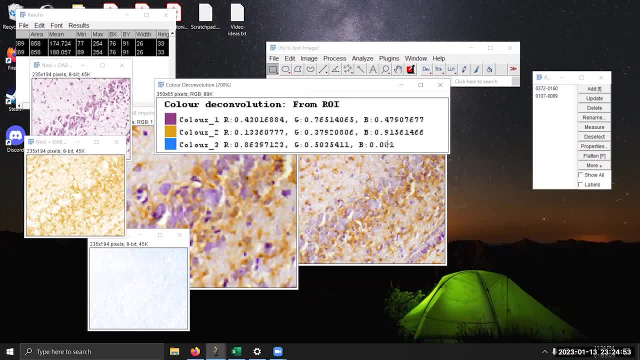 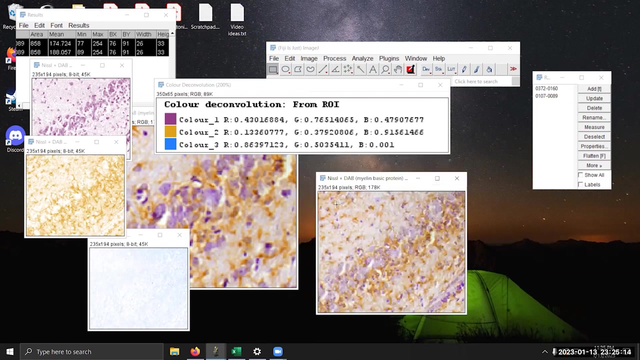 Blue color consists of this number red, this number green, this number blue. Now you can do color deconvolution for your second image, But instead you're going to use the values that you just obtained. So we can either type these in manually or we can copy paste them from itself. 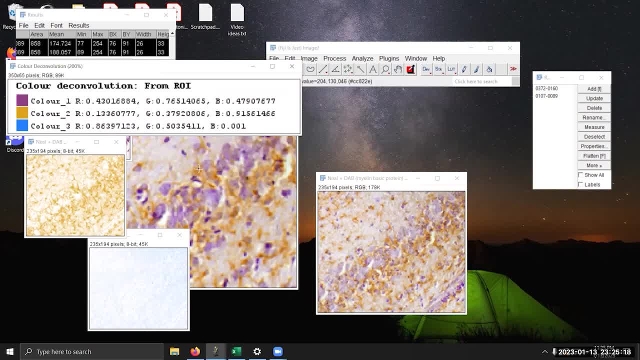 So i'm going to type them in manually, since we have them right here, Although i'll just sort of truncate them for simplicity. We go to image color Deconvolution. This time we will select user values. A new dialog box will pop up. 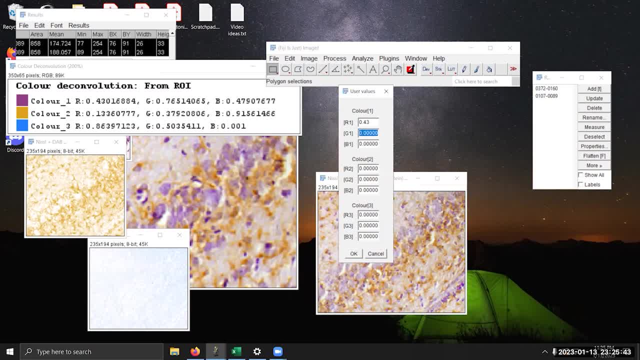 So i'm just going to type in 0.43, 0.765,, 0.479.. Next one: 0.1336.. 0.379., 0.392., 0.9156.. And then 0.86397.. 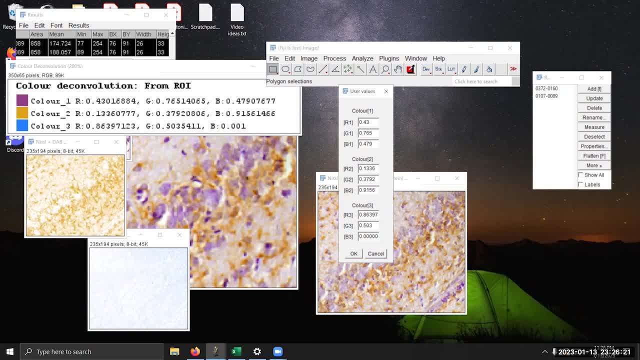 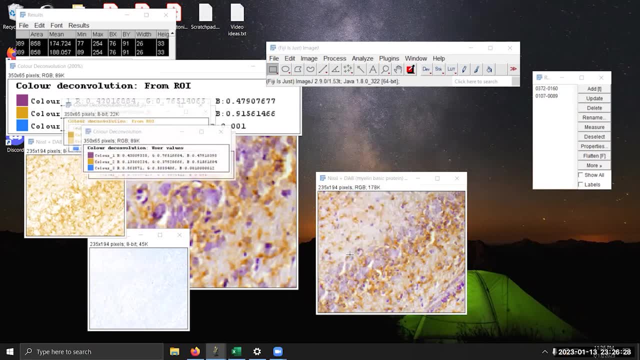 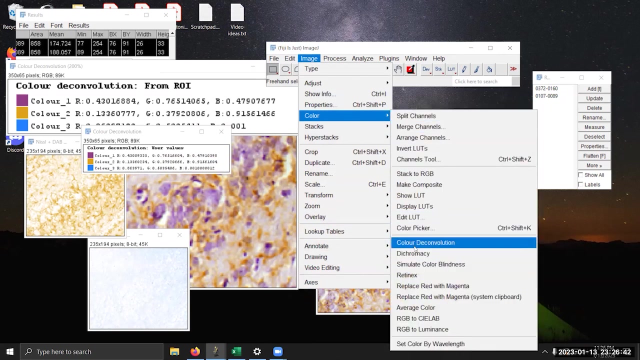 0.50354. And 0.001. And we will hit okay. Oops, I selected the color deconvolution box itself, So let's make sure to click on the correct window. Do that one again. Hopefully it saved the values. 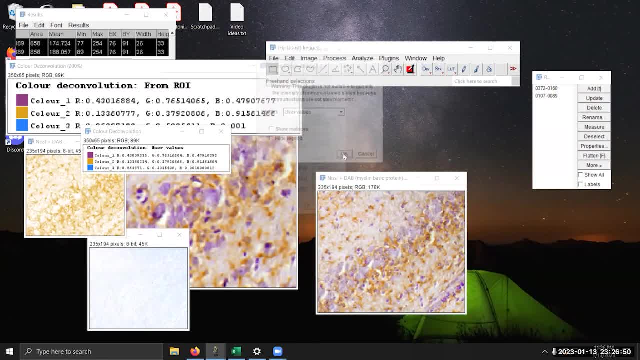 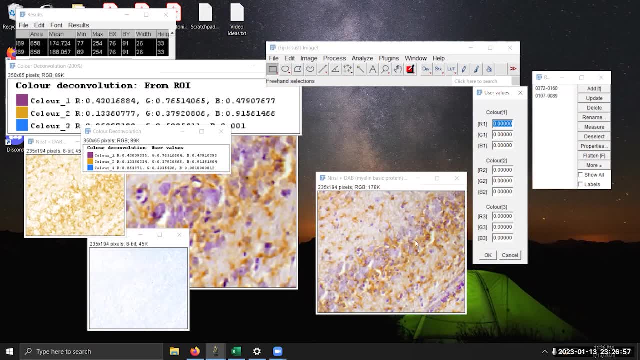 User defined. It did not, So i'm going to go ahead and plug in those values real quick once more. Okay, I will use the new tag to show the new values And then i am going to go ahead and log in, All right. 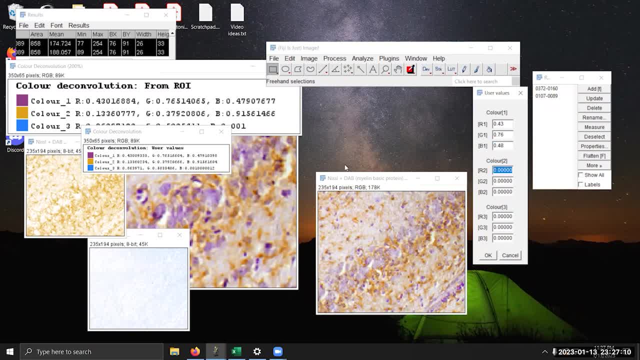 Let's see if the values are the same. I don't think so. Let me just see if it's the right one. 0.K. 0.679.. 0.916.. 4, 0.503, 0.001.. 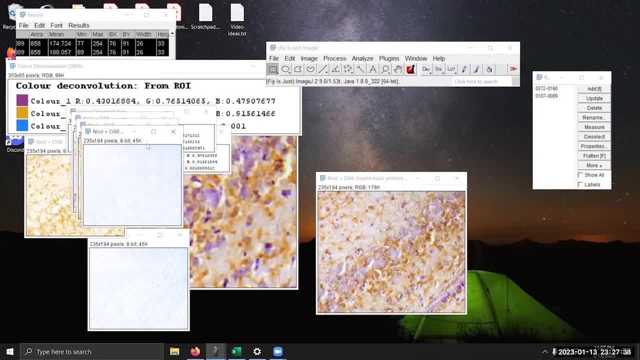 OK, There we go. Now we can visually compare the resulting color value channels split from the image. Let's finish up by selecting the areas of interest in each image and running the measure tool, as we did before. That's the measure tool, not the color histogram tool. 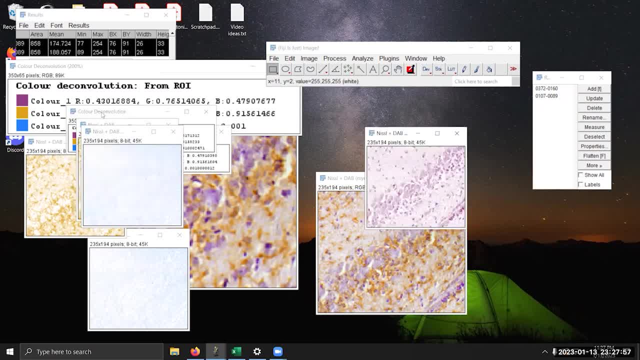 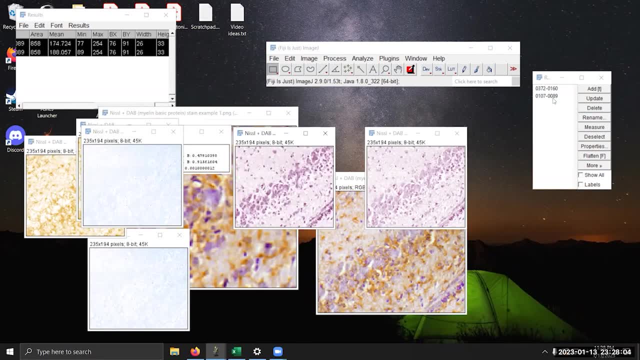 Specifically, I'm going to pick up the purple images here And I'm going to redraw it quickly with the ROI measurement tool And I'm just going to go into Analyze Measure and then Analyze Measure And we have our mean values here. 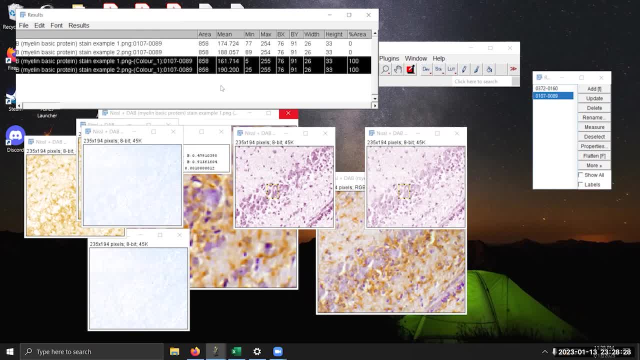 So I've copied these into Excel and we'll look at them in a little bit. Now I will skip Approach 4 for these images because, as we saw before, we will basically obtain the same values as we would have with Approach 1.. 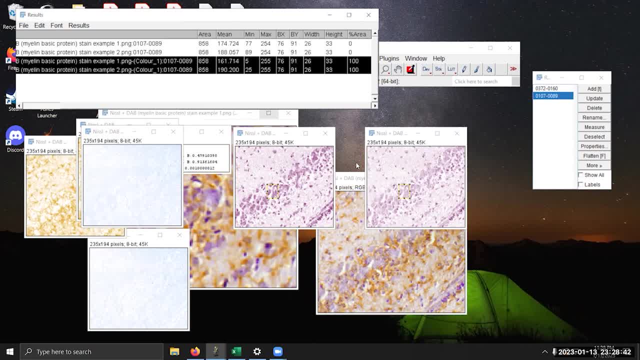 So Approach 4 on complex non-RGB stains my verdict more complicated than Approach 1, but with the same results. so I don't recommend it. So then we will do Approach 5.. Approach 5 on complex non-RGB stains: verdict. 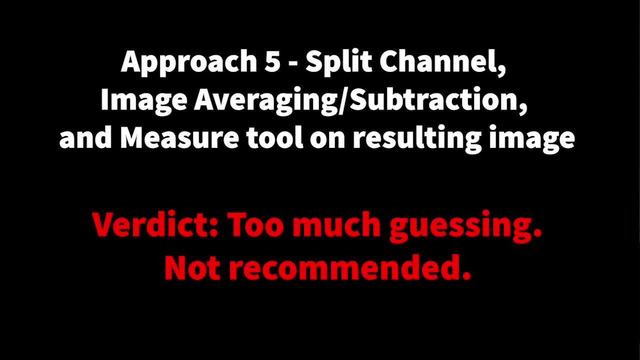 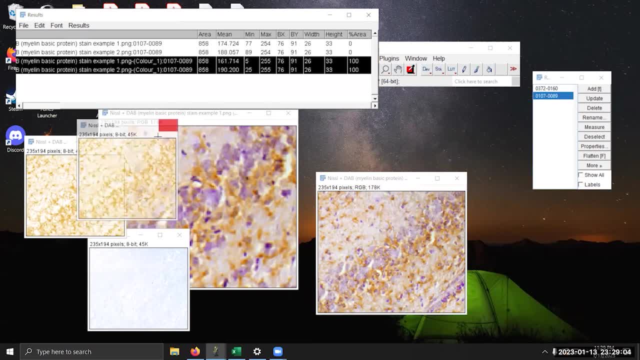 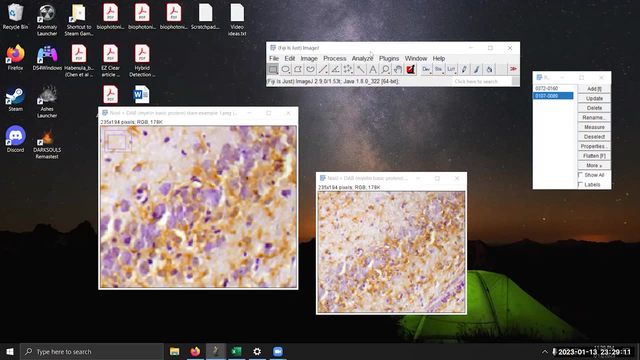 too much guessing, not recommended. So let's go ahead and set this up again. I'm going to close all these custom deconvolution images, Take each original image and split the channels as we've done before. So we go to Image Color: Split Channels. 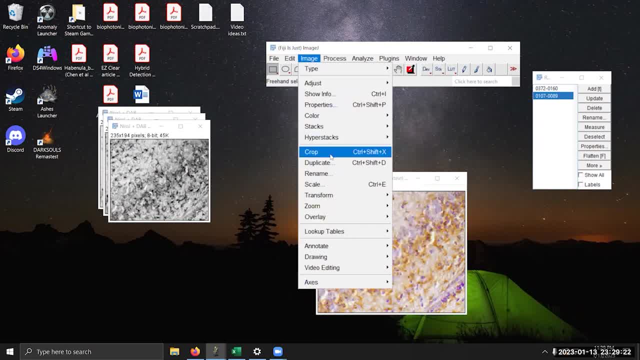 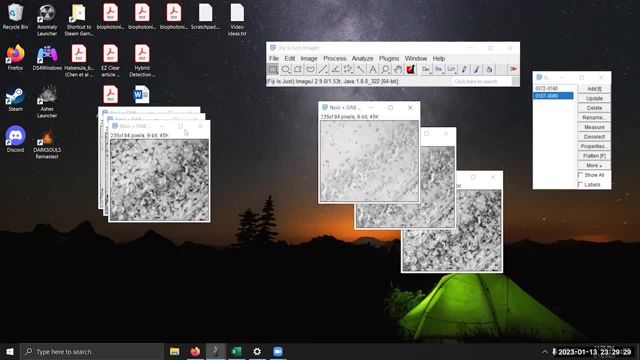 Do the same thing over here: Image Color Split Channels And we decluster them a bit. So we're going to do that. So we're going to do that a little bit so it doesn't get too confusing. Now this part will be tricky because the nistle stain. 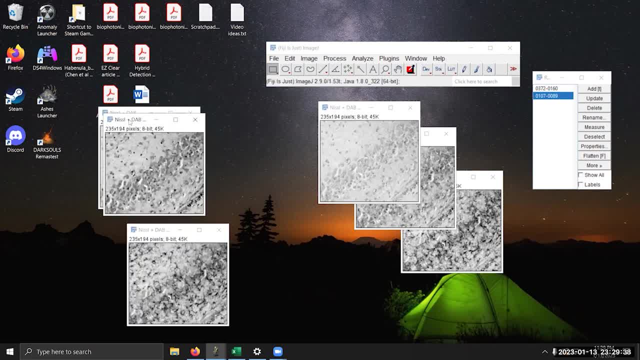 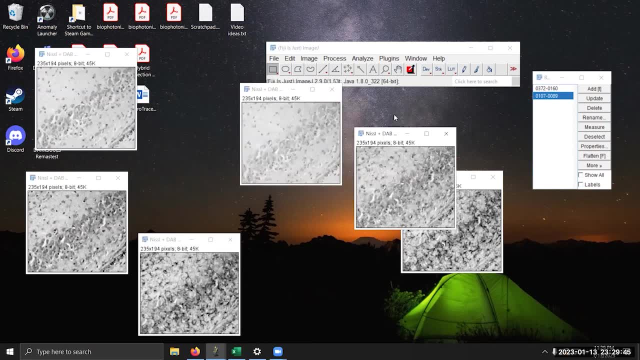 is purple, It's not specifically red, It's not specifically green, It's not specifically blue. So the closest approximation for purple that we can get is if we were to combine red and blue channels. So for the image calculation aspect, that is actually what we'll have to be doing. 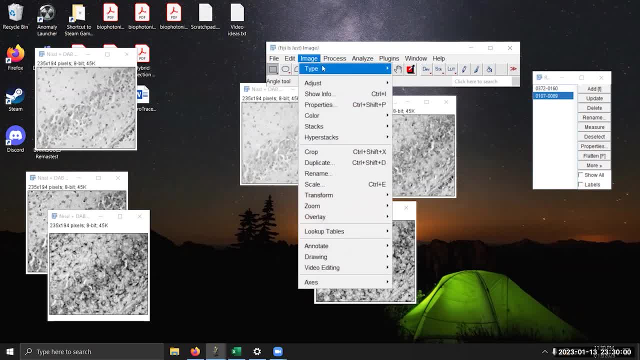 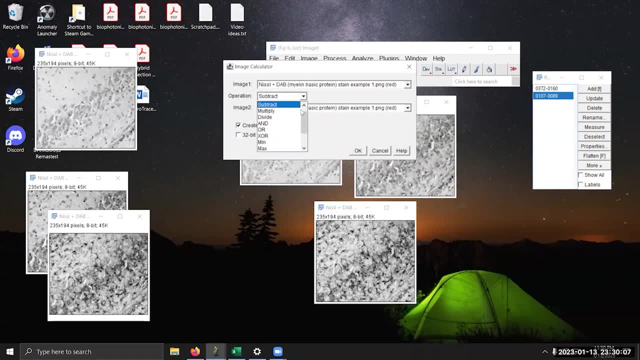 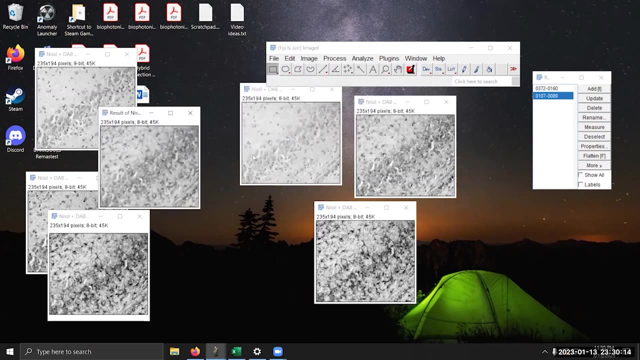 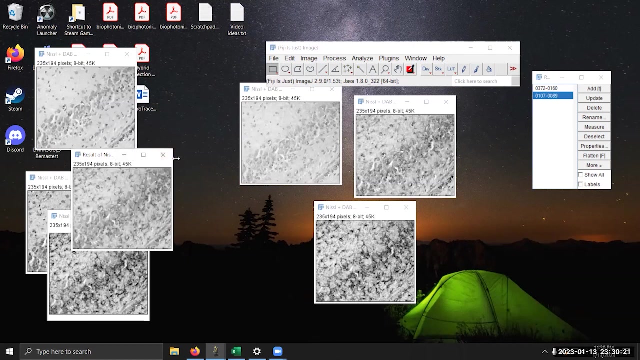 So I will do that with the first set of images here, Process Image Calculator. We will take the very first image- Function is Average, And then blue. for the second image It will create a new image over here And from the resulting image use that calculator again. 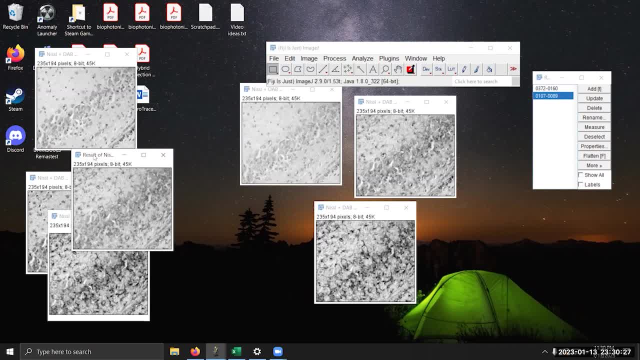 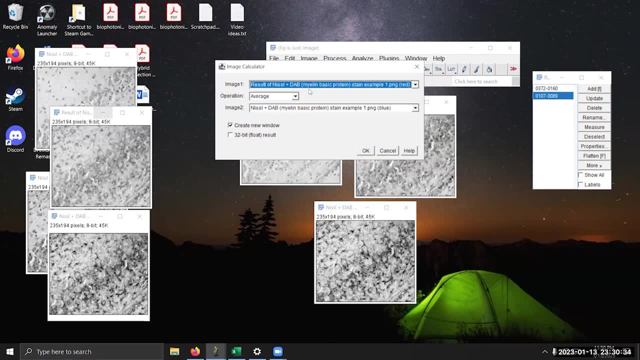 to subtract the green channel from this. So we go into Process Image Calculator, We take Result, Image Function is Subtract And then we select Example 1, Green, And we hit OK. So this is the final product we're interested in. 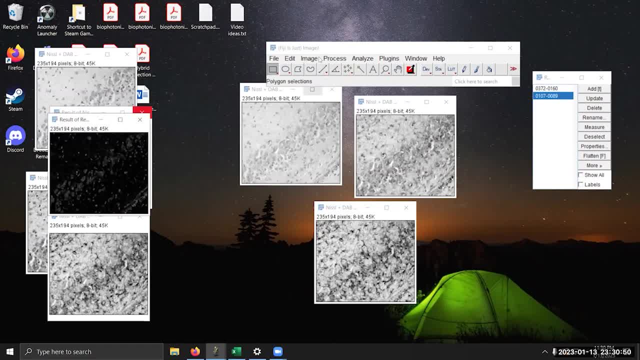 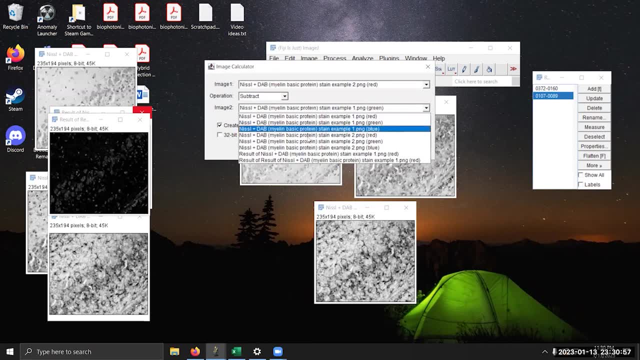 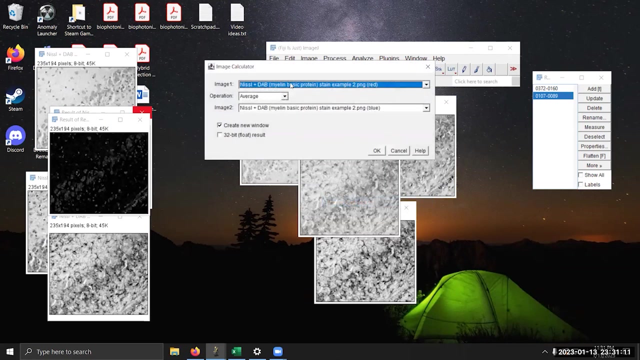 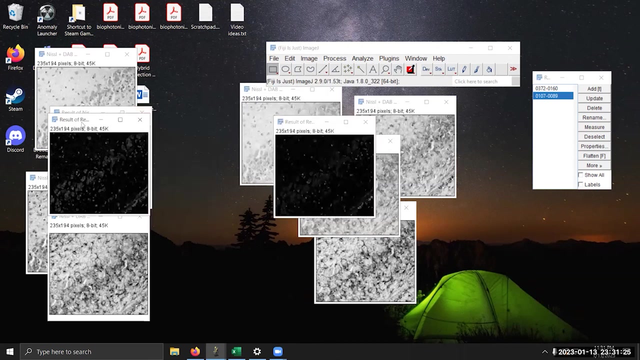 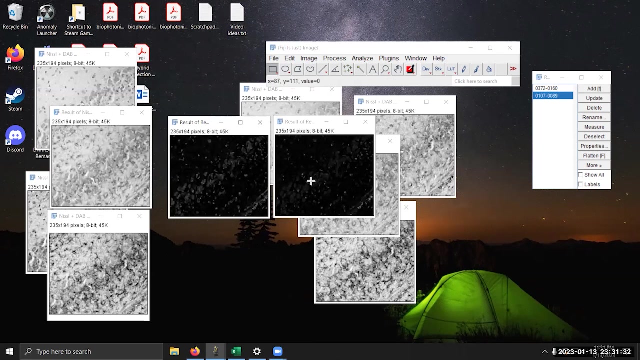 We'll then do it all over again with the second set of images for the faded stain. OK, OK, So now we have these final resulting images side by side. We can definitely see the difference between one being more dim than the other In these final resulting images. redraw your selections. 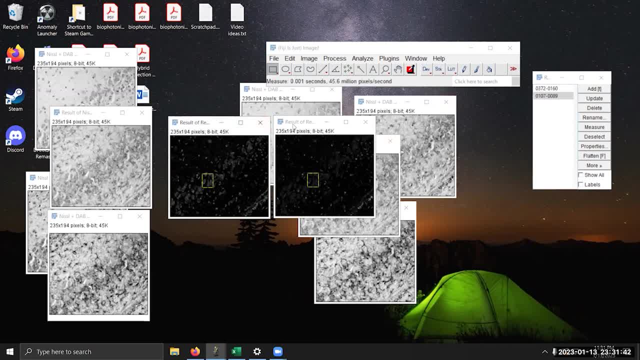 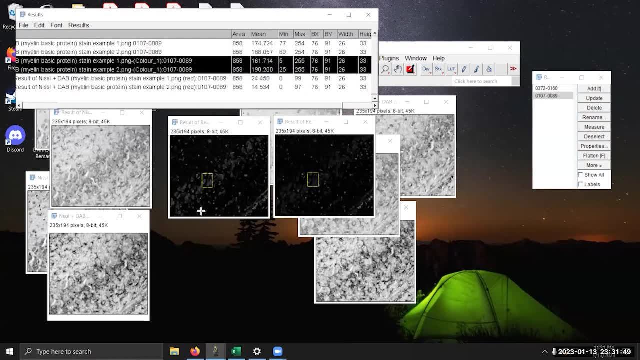 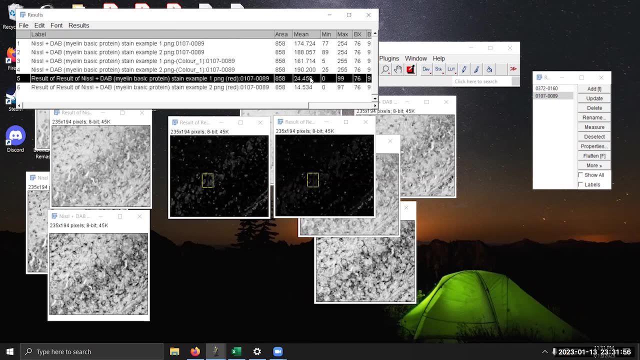 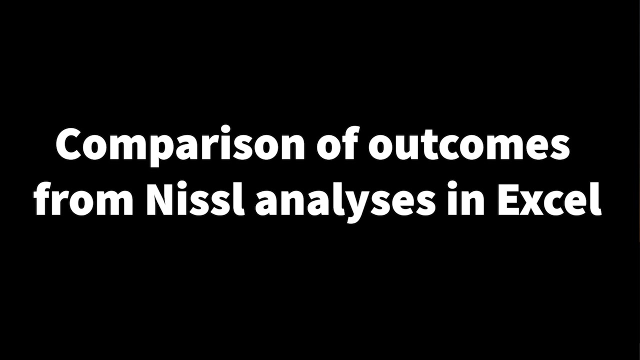 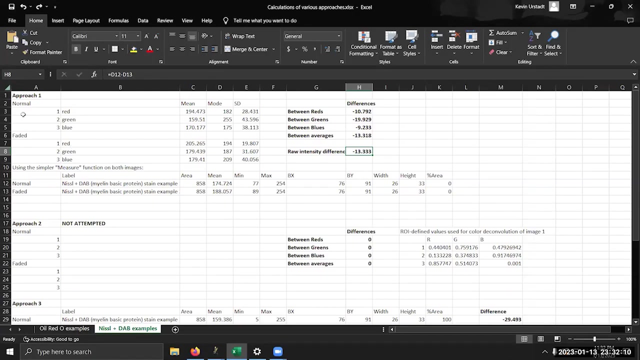 and use the measure tool accordingly, And so we again have the values down here. So the mean values are displayed right here. Let's again compare the values obtained from these three methods. I applied to this set of images here, So in the second tab I have here values. 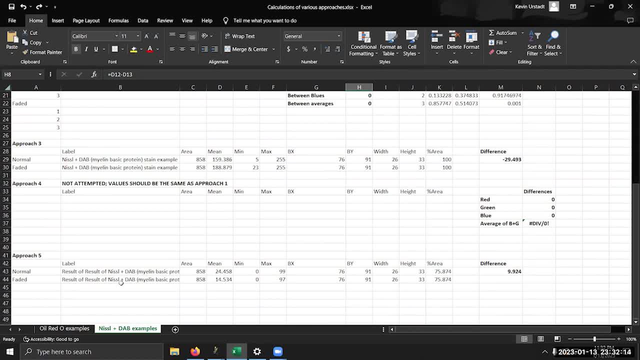 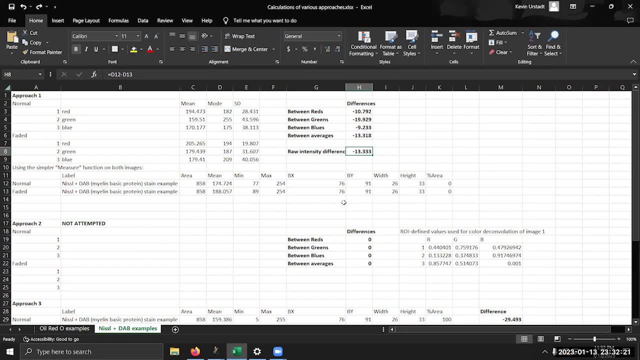 obtained by Approach 1,, Approach 3, and Approach 5,, again having skipped Approach 2 and 4.. For Approach 1,, we see that the average intensity difference of the selected areas in the multicolor images is rather small in the scope of a 255 color range. 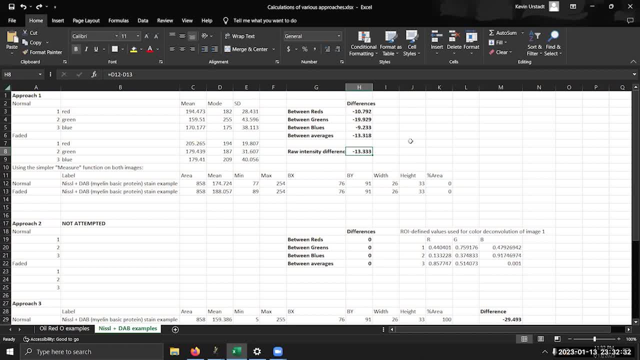 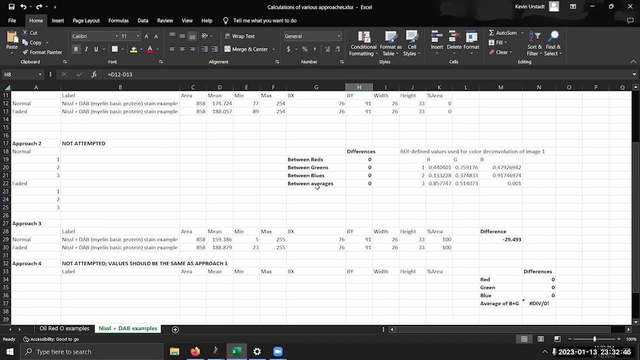 We basically only see a difference of 13 shades out of 255 possible. Meanwhile the color difference is rather striking. It doesn't look quite that subtle, So this seems like a lowball estimate to me. For Approach 3, where we use custom color, 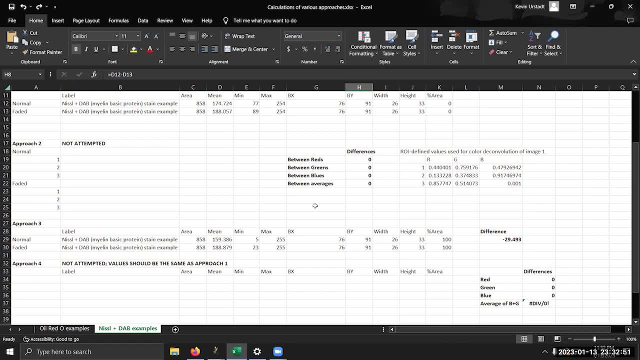 deconvolution approach. the intensity value that we were given, or the difference of the intensity values, is 29.. That seems a bit more believable because there is a notable difference. It's 30 shades difference in the level of purple. 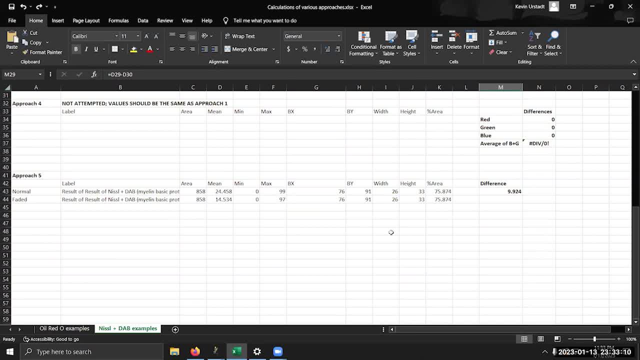 And then for Approach 5,, when we use the channel splitting and then image calculations, we obtained an intensity difference of 9, which, based on what I mentioned earlier, again seems far too small. OK, So if you are using a stain that is not easily split, 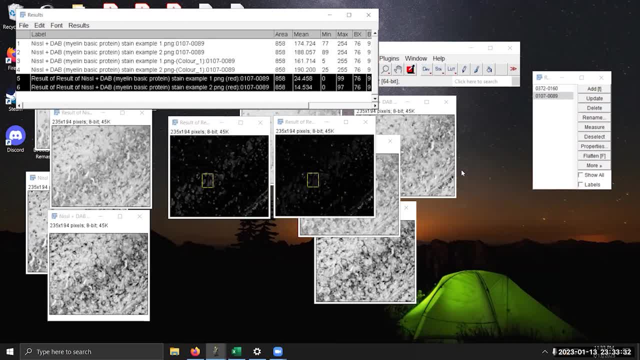 into red, green and blue. I strongly recommend going with Approach number 3, in which you determine your own values for color deconvolution with an example ideal stain image and then use those values to deconvolute other images with the user values setting. 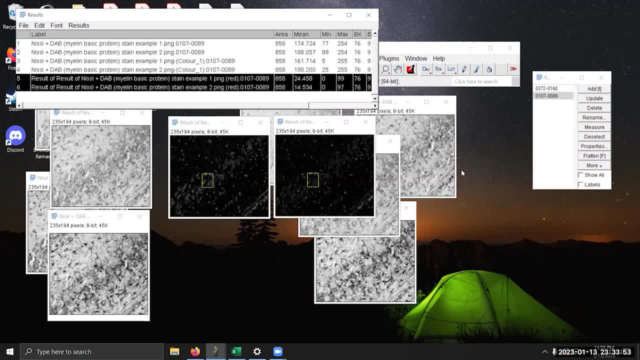 Then apply the measure function on the channel of interest within your selected region of interest in order to get the most accurate color values. The other approaches that we've tried just can't grapple with these types of stains appropriately and thus are liable to give you misleading information. 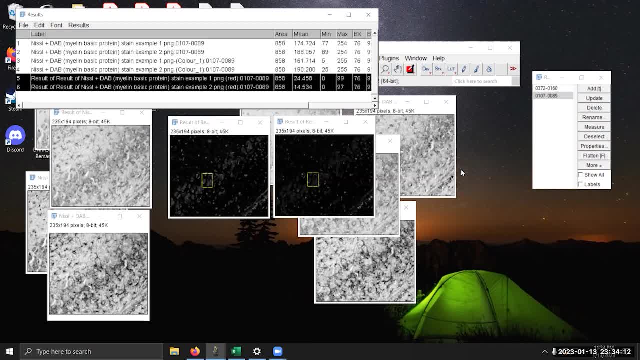 I would say that the other approaches are not entirely inaccurate, but they definitely give less precise information than Approach number 3.. Regardless of which approaches you use, it's important- I would say even extremely important- that you remain consistent in using just that approach. 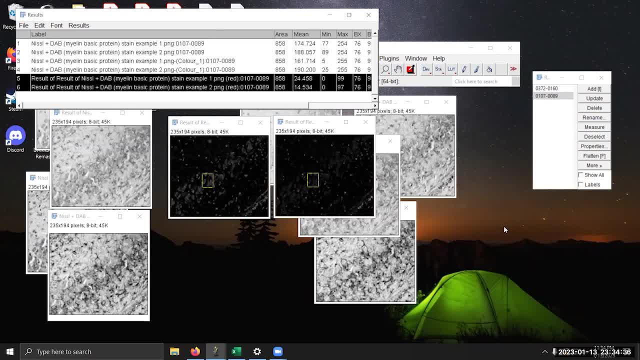 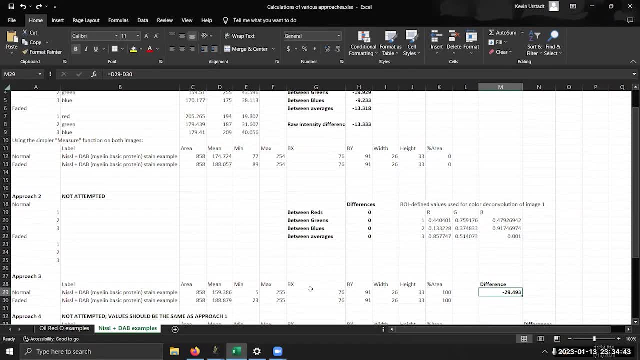 throughout your whole experiment. You do not want to be changing your approaches, because that will change your values dramatically. as far as what we've seen, There's a steep difference between, let's say, values like 13 versus 30, or worse yet.